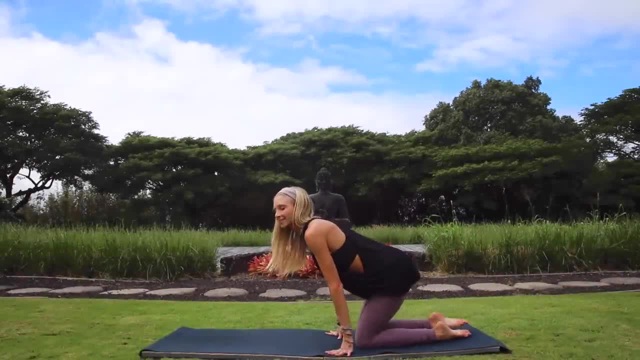 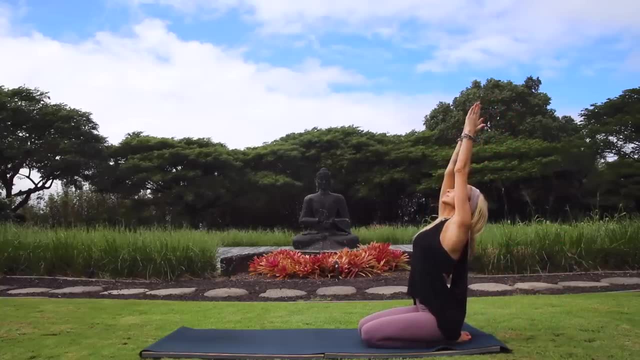 All right, friends, we're going to begin today in your child's pose, So go ahead and sit to the very back of your mat. You're going to reach both arms all the way up to the sky, Take a deep breath in and then, as you exhale, go ahead and release your body all the way forward with your chest. 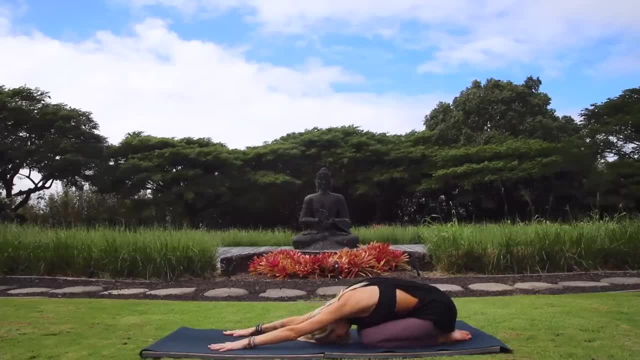 releasing over top of your knees, Allowing your forehead to come all the way down, and just release your body all the way forward, with your chest releasing over top of your knees, Allowing your forehead to come all the way down, and just breathing deeply here, Taking this opportunity to connect your body with your breath. 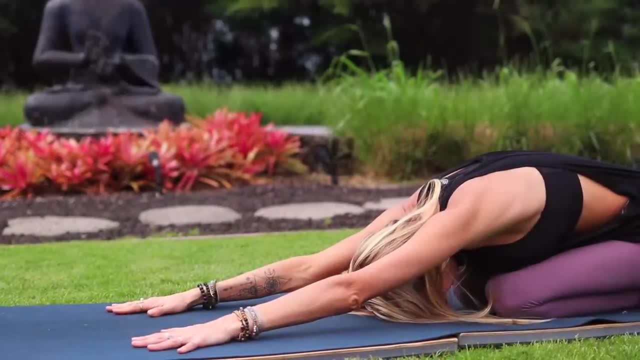 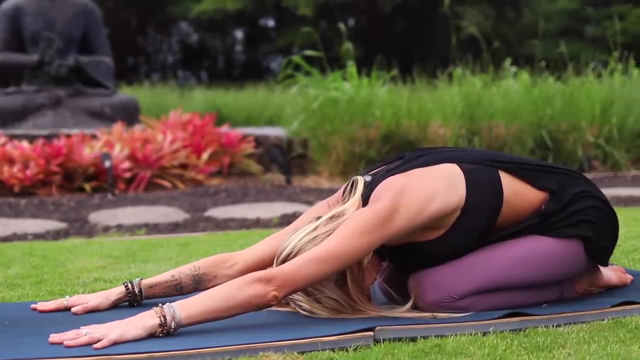 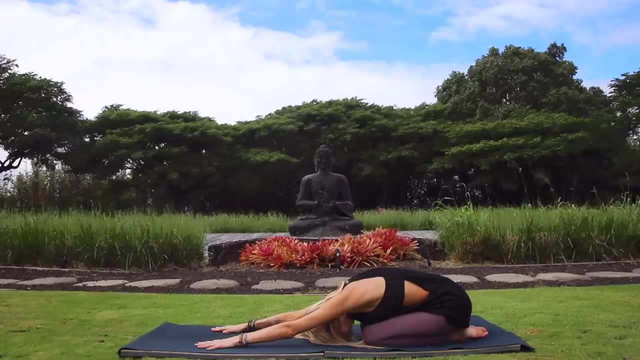 Inhaling gently into your nose and exhaling softly through your mouth. Become aware of your body doing a quick body scan here. Notice where you feel the tension and stiffness and resistance and once you've found the particular spot, breathe a little bit more oxygen into that. 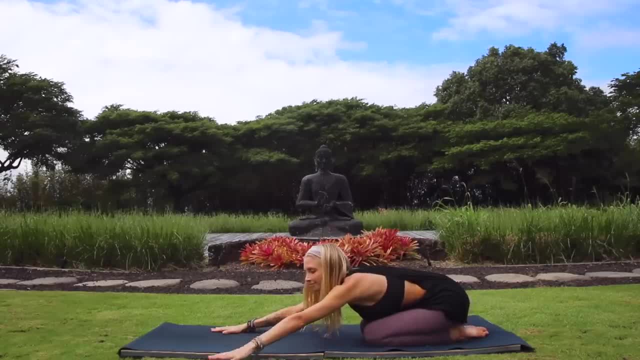 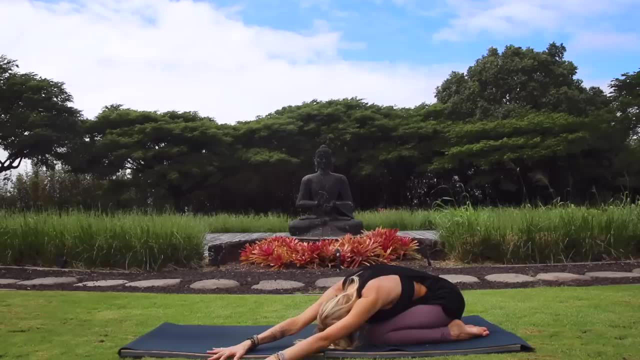 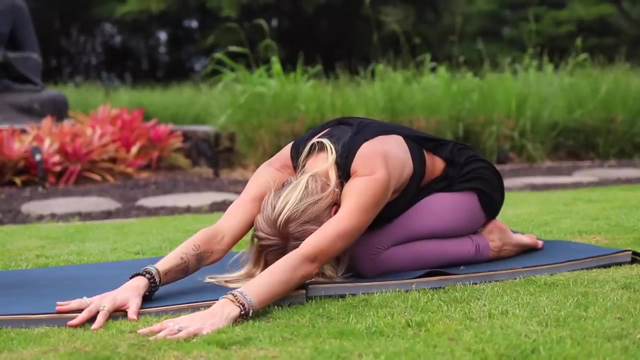 area of your body. Wonderful. Now, from here, stay in your child's pose and just simply bring your hands to the very left side of your mat. So now you're reaching, going a little bit deeper into the right side of the body, and same thing. just continue to breathe, Feeling that gentle stretch, taking it as far as you. 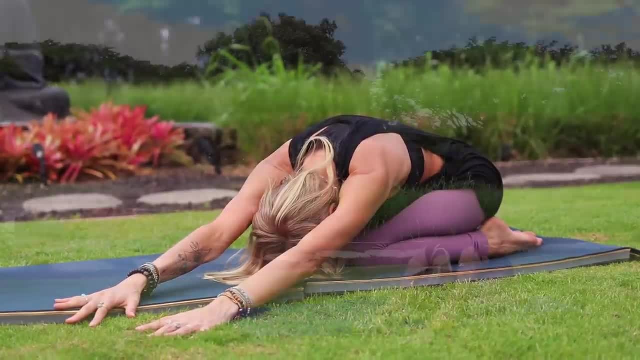 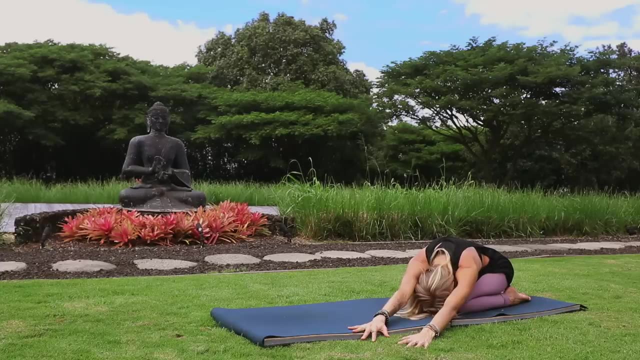 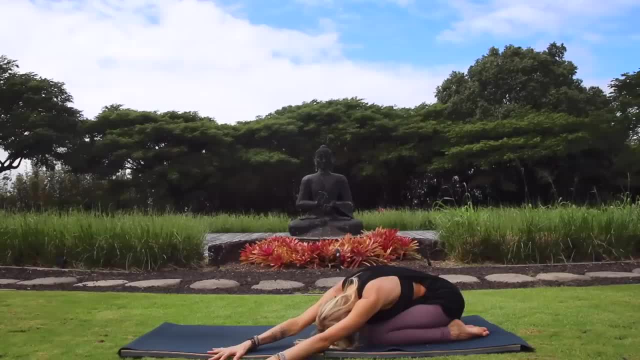 If you have an injury where a child's pose does cause pain, you can do this. If you have an injury where a child's pose does cause pain, you can do this. I would like you to avoid child's pose for today's class. 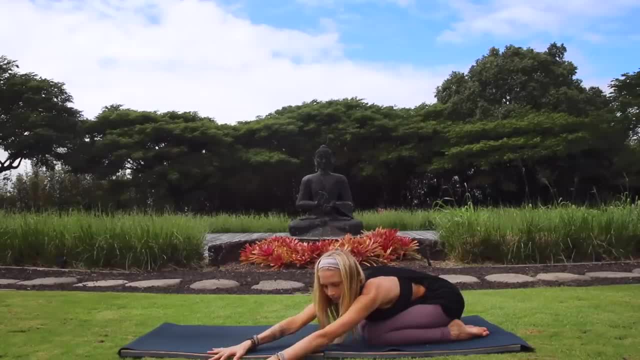 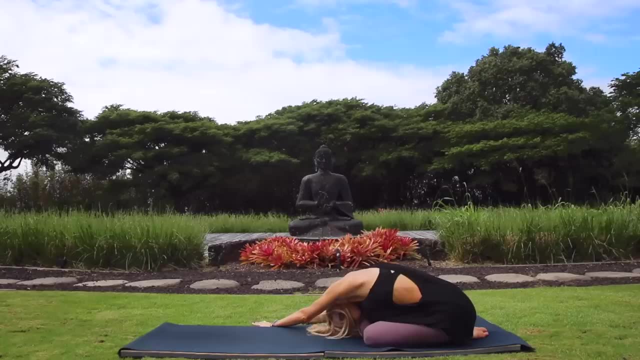 You can simply sit up straight and wait until the next posture comes. Awesome, Let's go ahead and take it to the other side. So same thing. now, reaching both hands to the very right side of your mat, Your hips are staying exactly where they are. We're just gently. 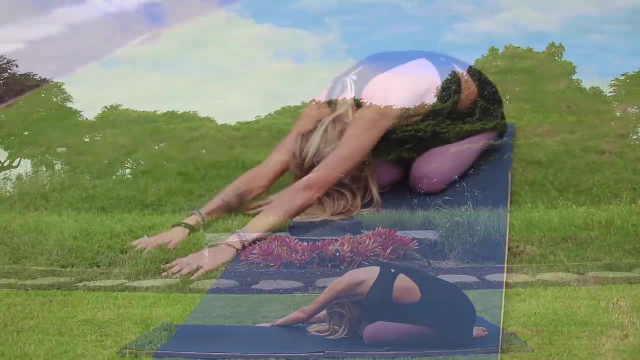 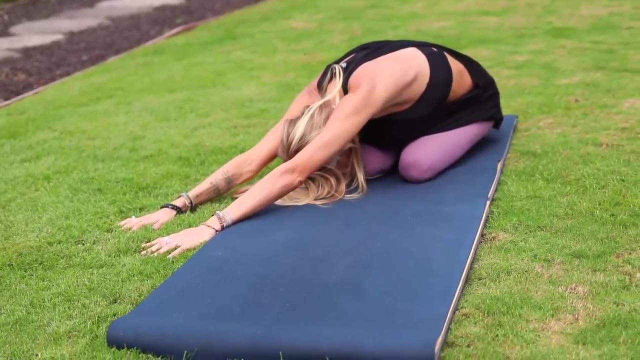 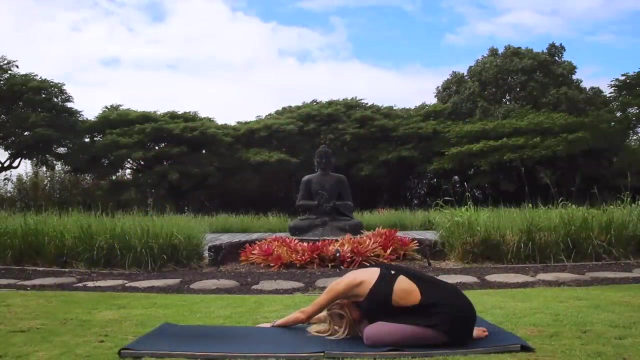 folding from the side, breathing into the left side of your body now, Breathing deeply, allowing that forehead to release. Be very conscious of how you feel here. Where do you feel resistance? Welcome more oxygen into any area of your body where you feel that tension and let go. 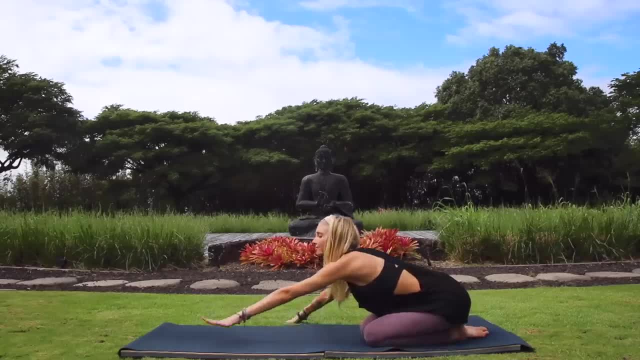 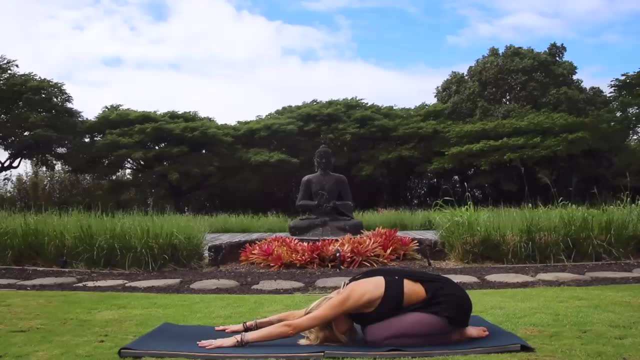 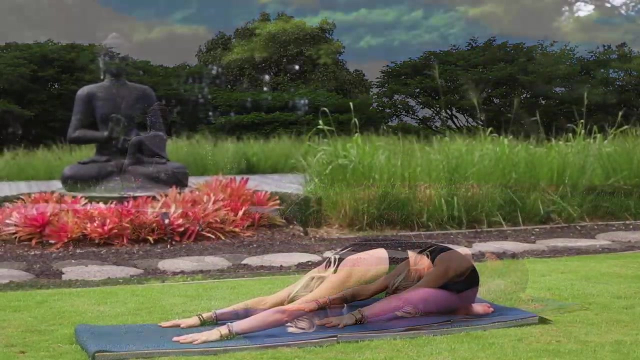 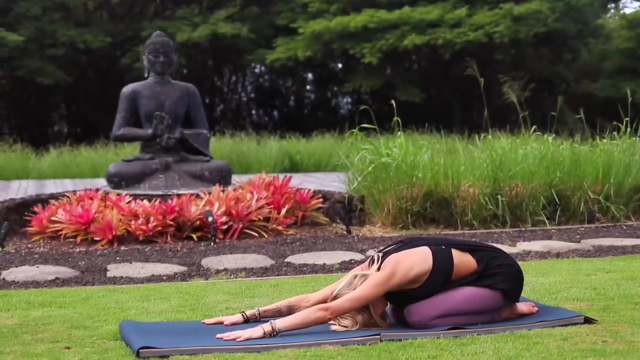 Wonderful. let's slowly come on up. Bring yourself back to that center position. child's pose Deep breath in reaching those arms forward, feeling a gentle stretch through the shoulders here as well, Great job. Allow those hips to sink close to the heels. a very gentle release on the back here. 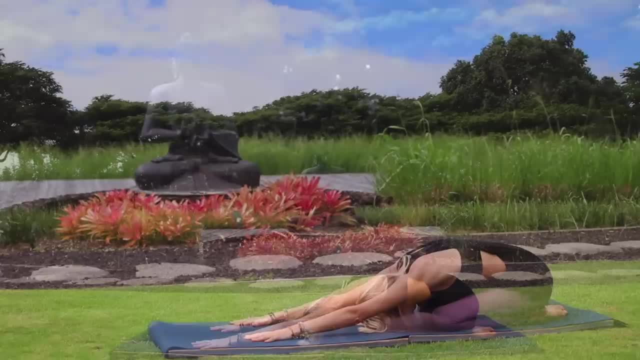 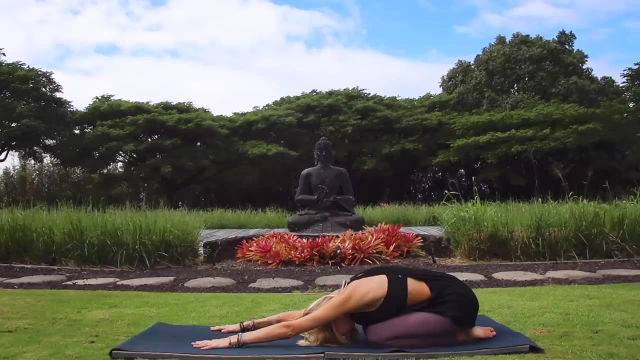 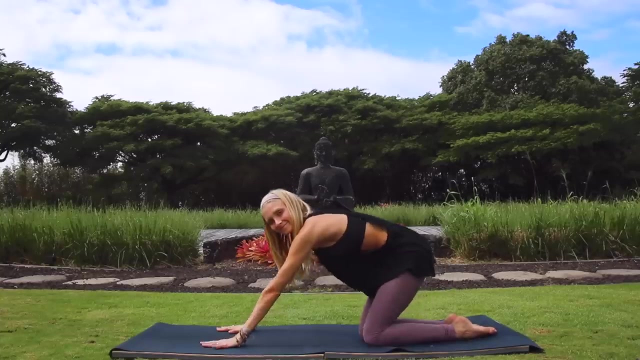 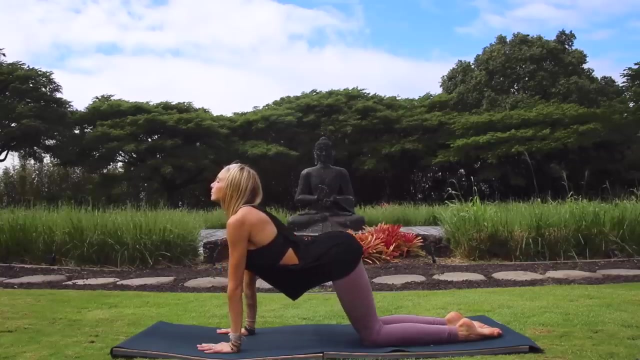 Deep breath in, exhale out. Another deep breath in, Exhale out. Now, as you exhale, come on up to your all force position. We're going to begin with cat-cow, welcoming some movement into the spine: Inhale, arch the back and then, as you exhale, round the spine and bring that chin into the. 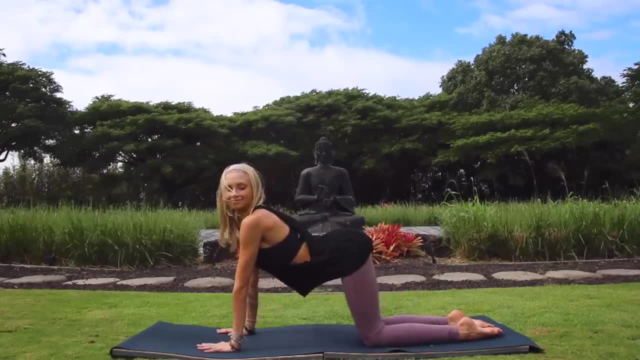 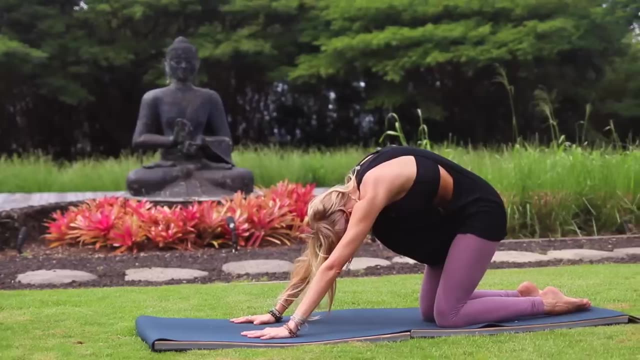 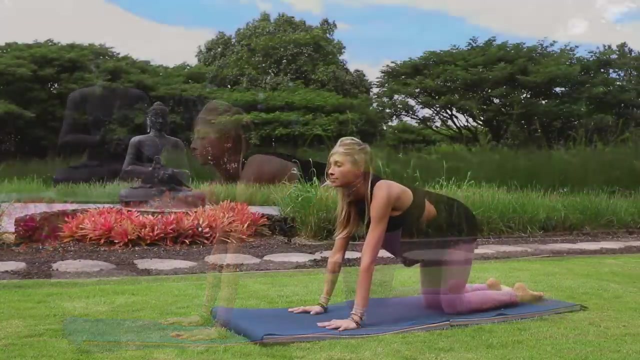 chest, Inhale, arch the back and then exhale: release. Now, if you do suffer from any herniation in the spine, make sure you come back into neutral position and don't round the spine here. Just arch the back Again. come back to center. 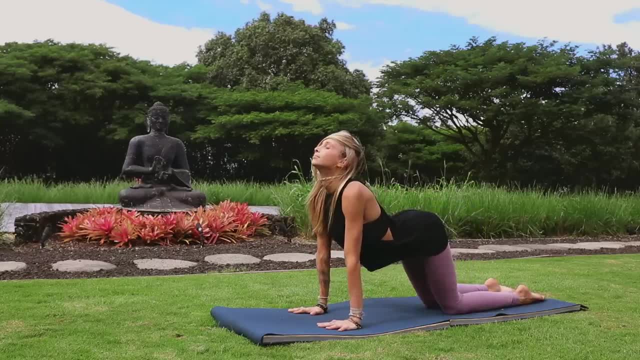 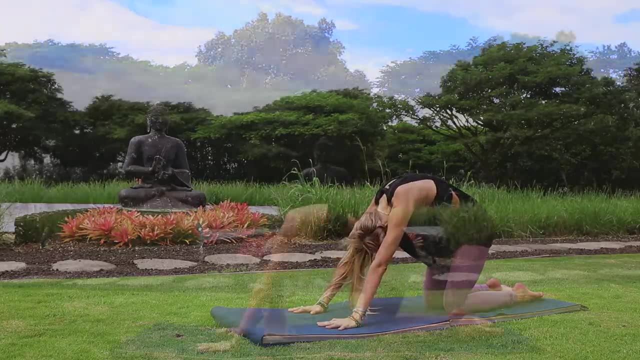 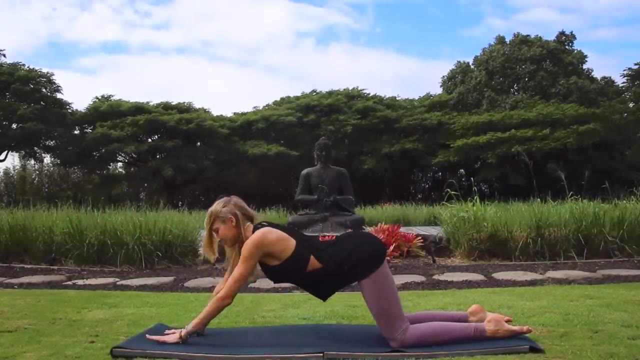 Be very gentle with the spine, Listening to your body. Deep breath in exhale Round, Bring the chin to the chest And then step back with your knees slightly On your inhalation. you're going to bring both hands to the very front of your mat and 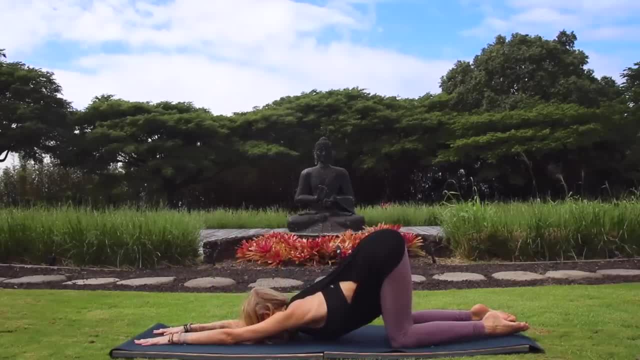 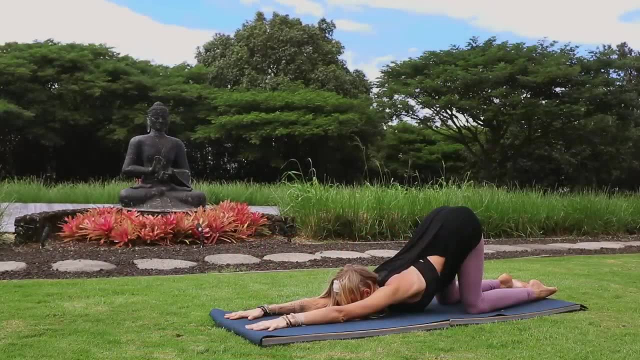 go ahead and release into the puppy posture, making sure the hips are staying on top of the knees. Your elbows are extended. Now you can choose a couple of variations here. You can either keep your forehead grounded or, if you do, feel, comfortable in this posture. 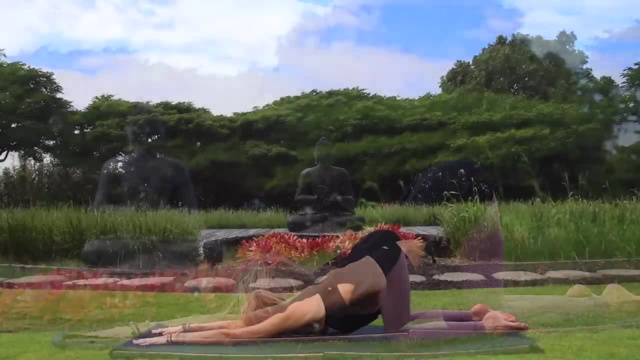 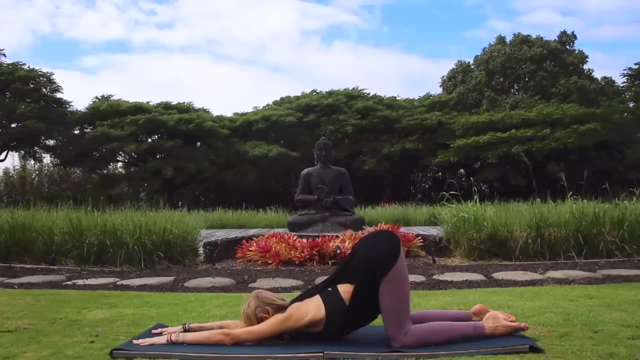 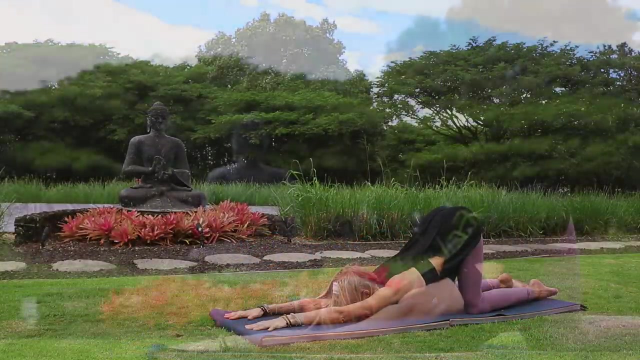 and you'd like to go deeper. bring your chin towards the floor, So bringing your gaze up towards your fingertips, allowing your chest to come down even further towards the ground, welcoming a deeper opening, and stretch along the upper back Deep breath in, exhale out. 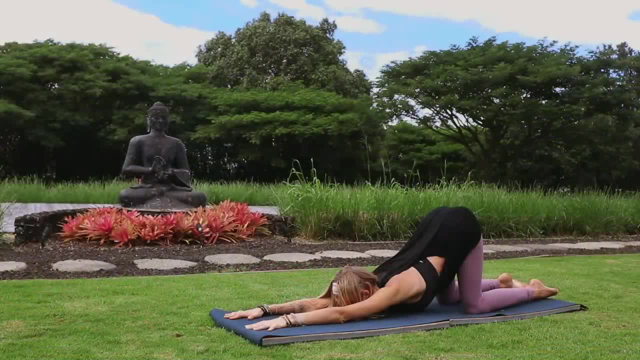 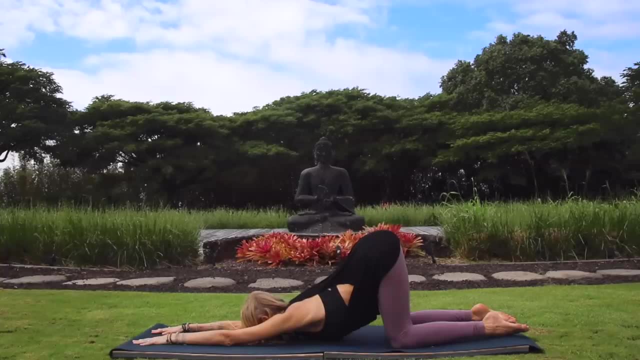 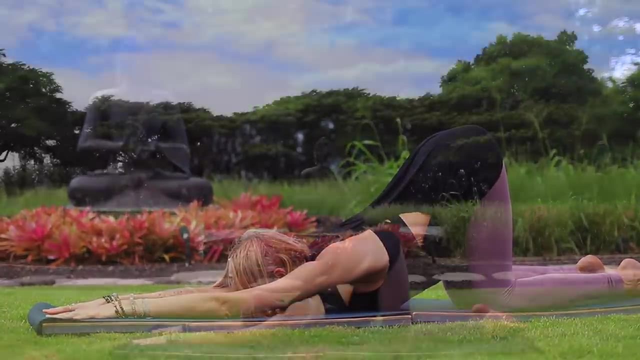 Just allow yourself to stay present with your breath Throughout our practice. today we're going to be holding many different postures, So while you stay and breathe, focus on your mind sending positive energy into your body. Let's bring our weight over onto our elbows. 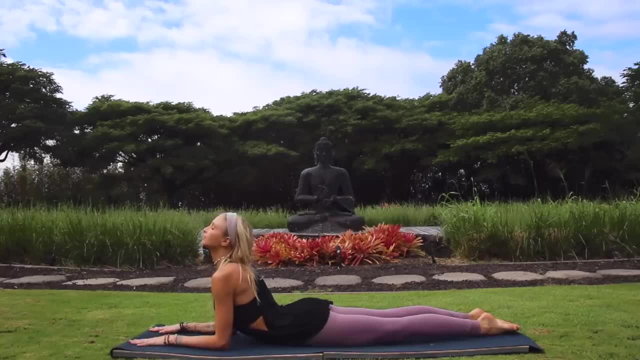 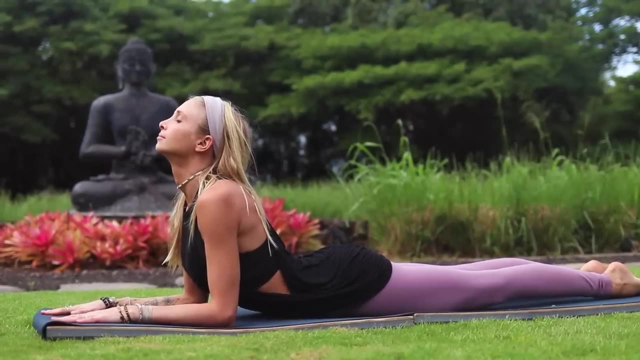 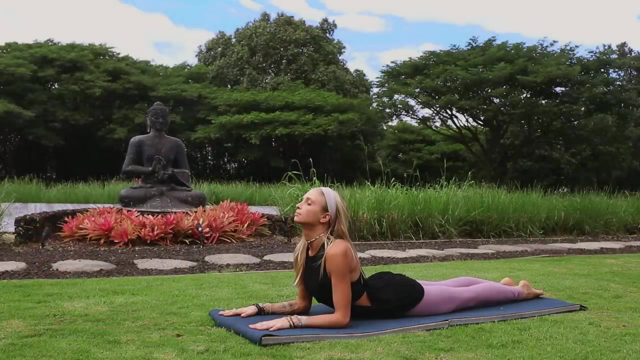 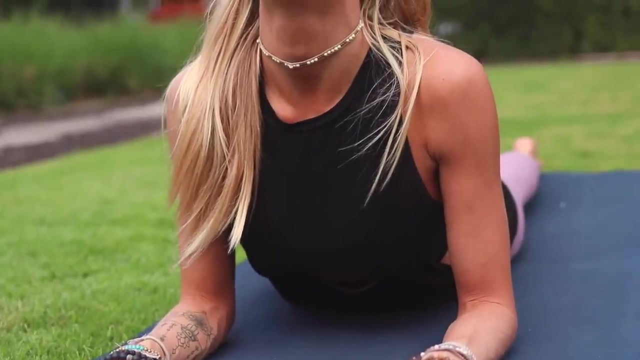 Put the hips to the floor. We're just going to take a baby cobra here, so stay on your elbows and then open through the chest, Drop the shoulders away from the ears and look up towards the sky, So really opening here through the heart center. a very gentle back extension. 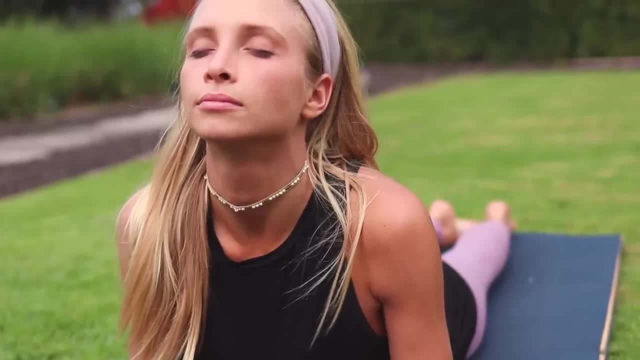 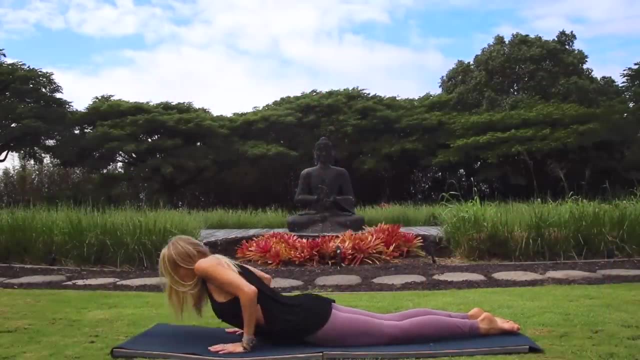 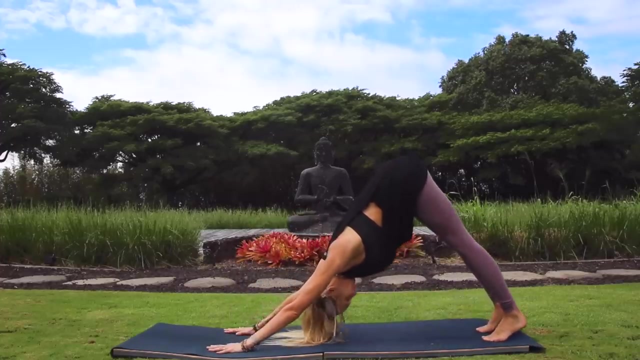 Deep breath in Exhale. Just stay here. Feel free to close your eyes. Coming back down now, Forehead to the floor, bring yourself up onto all fours. Let's tuck the back toes and then bring your hips all the way up towards the sky, into our 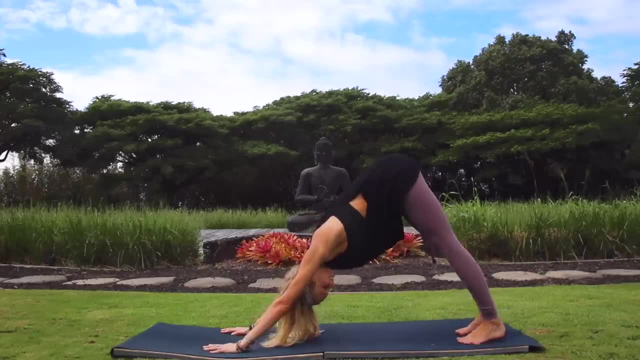 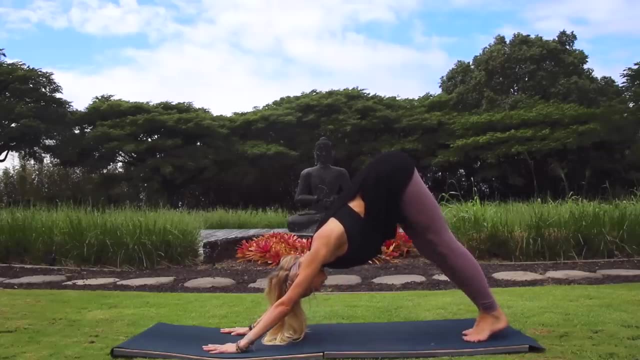 downward facing dog. Now feel free to walk out your dog here if you need to, or bend the knees if you have a little more tension in the hamstrings, eventually working your way over to a straight knee position. So again, just cater for that. 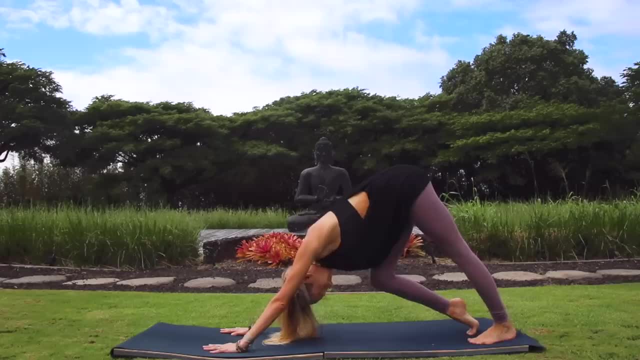 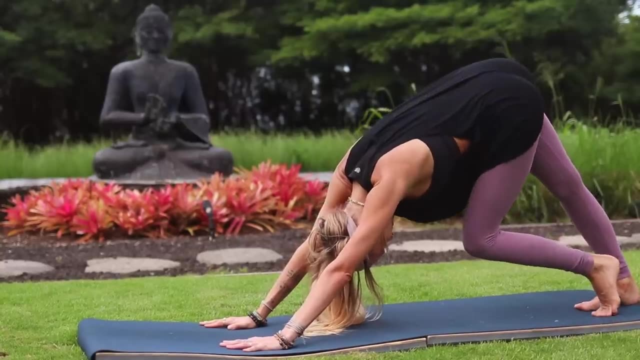 Stay here, Just stay here. Consider this posture to your own level. Spread those fingers wide, Walk out your downward dog to add a little movement here. This is our very first downward dog over practice, so your body's going to feel a little bit. 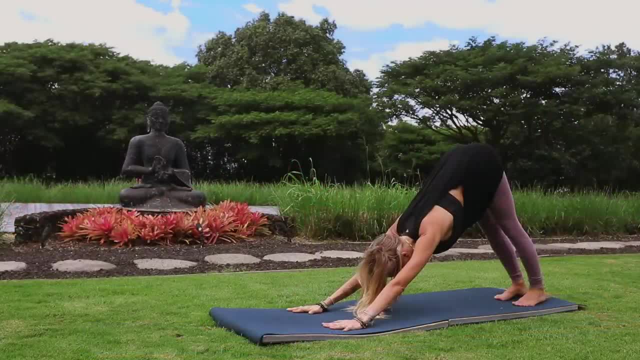 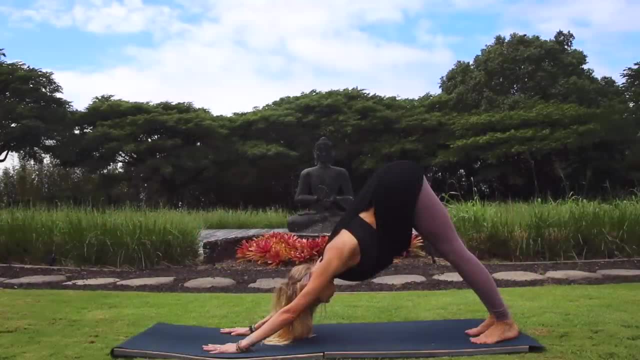 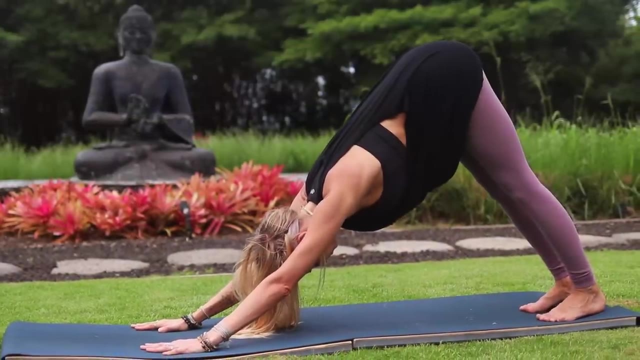 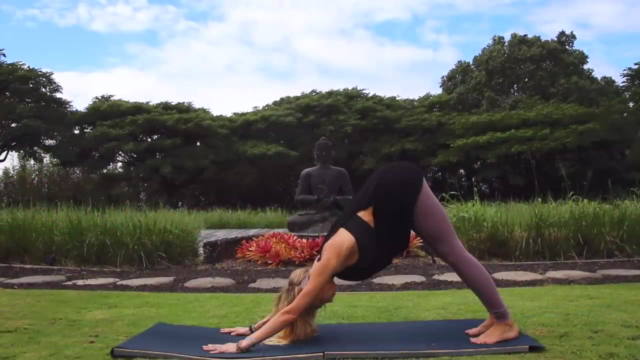 more stiff right now. Once you get into your downward dog position, just allow that sternum to fall towards the mat. Deep breath in, Exhale out With each exhalation, allowing the heels to come closer towards the mat, Working on getting both of your knees straight here. 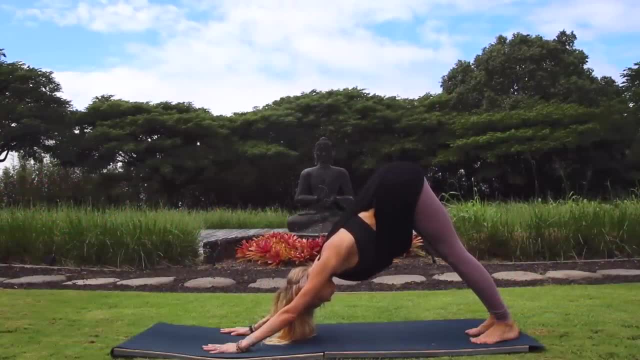 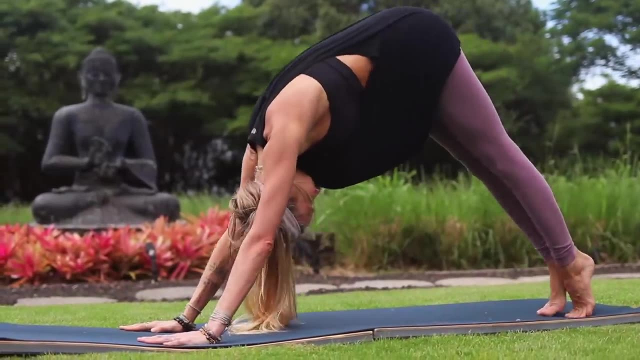 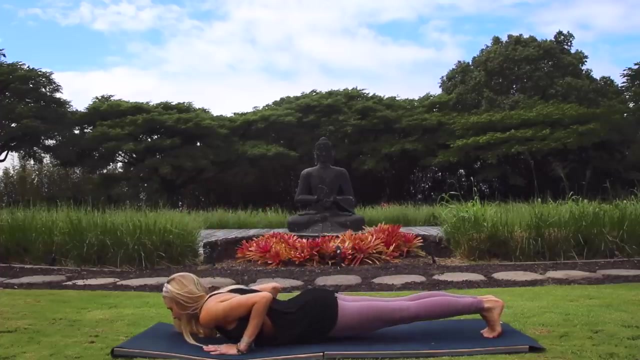 Tailbone is pointing up towards the ceiling. Take another deep breath in Exhale, Just stay there And then begin to slowly round through into plank position. You're going to drop down into a chaturanga, or more like a pushup hovered above the floor. 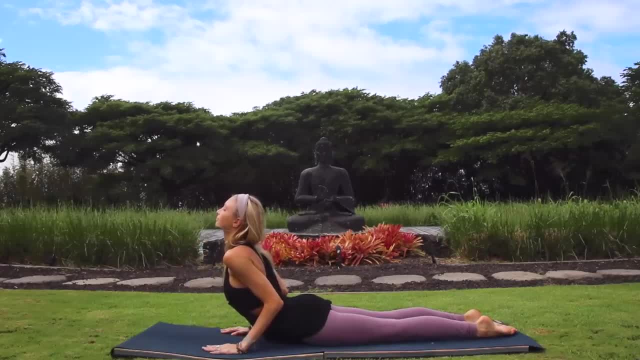 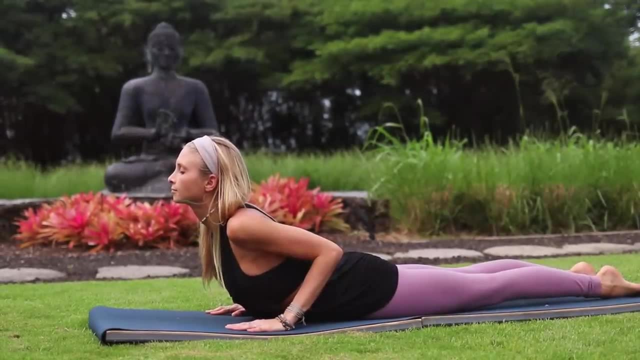 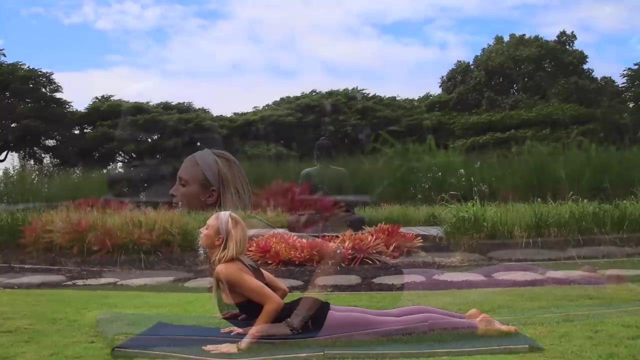 And then drop the chest to the mat, Opening into that baby cobra again, And then bring yourself out Holding here and just breathing. Notice how this posture feels on your body. If you'd like to go up a little bit higher, you can. 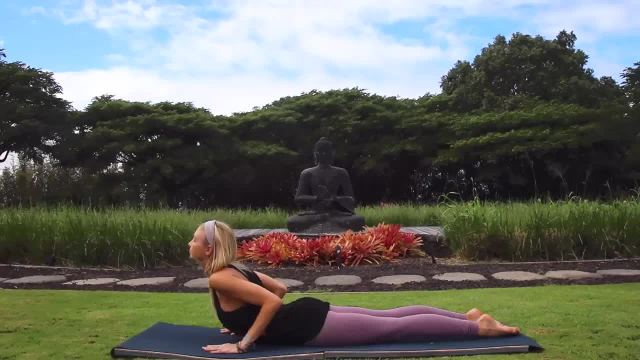 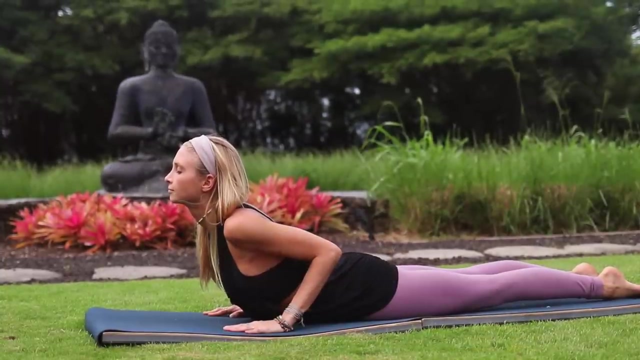 Or stay low, like we did in the very beginning of the class. Just a gentle back extension here. Keep holding One more deep breath in, Keep squeezing those back muscles, lifting that chest off the mat, Strengthening the back area here of your body. 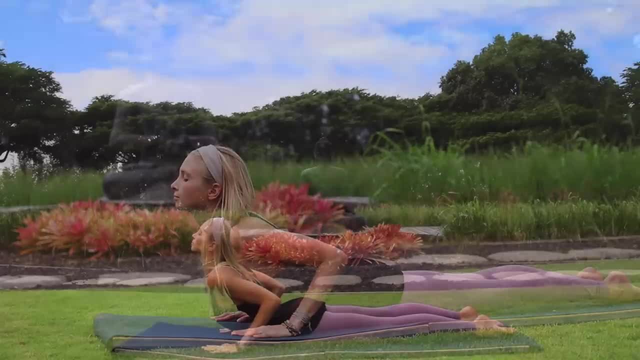 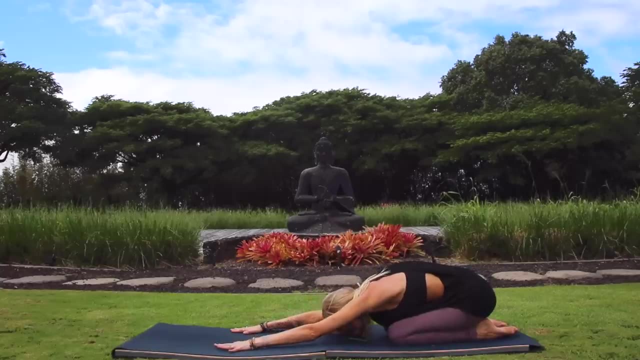 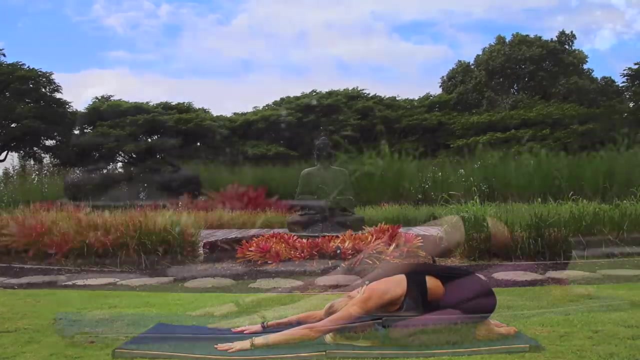 Deep breath in again, Lifting a little higher if that's comfortable for you, And then exhale. push yourself back into your child's pose, Rounding out the spine in the opposite direction, Stretching out the muscles, gently Reaching with the fingertips to the front of your. 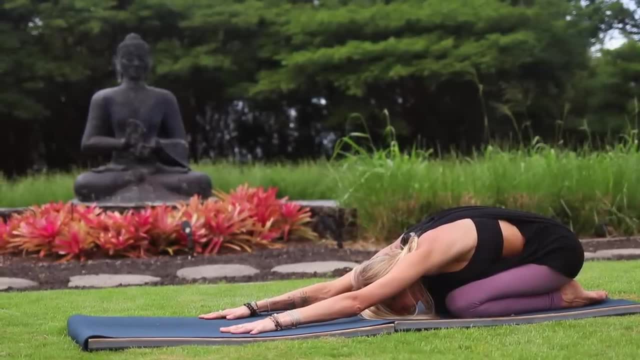 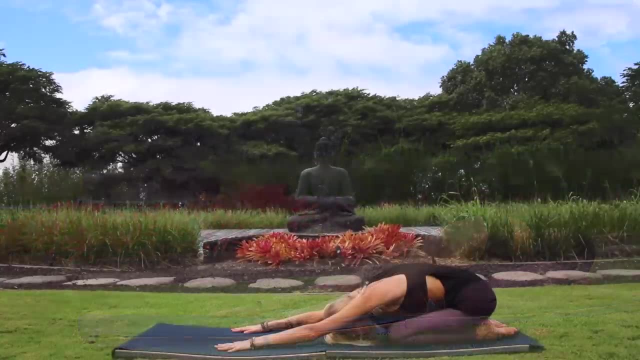 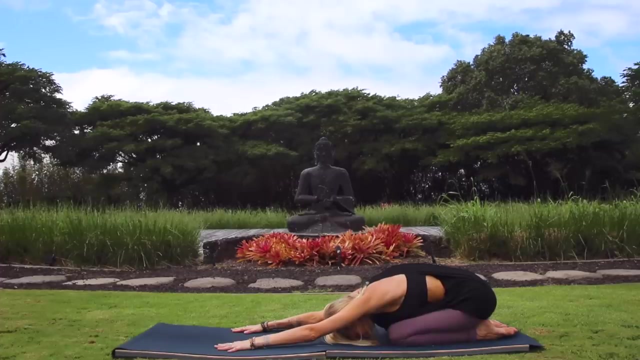 mat Lengthening through the shoulders. Take another deep breath in Exhale, allowing yourself to surrender over top of your legs. Stay present with your breath. Be patient with your body. Wherever you are is exactly where you need to be. 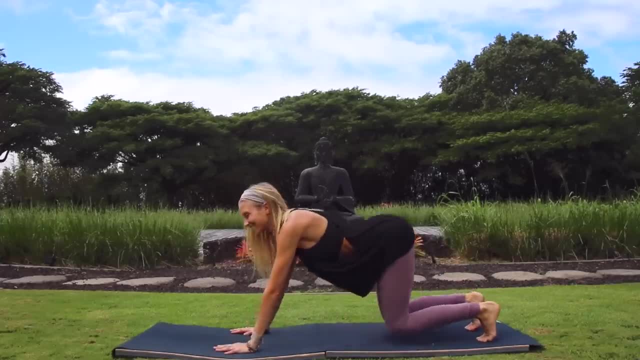 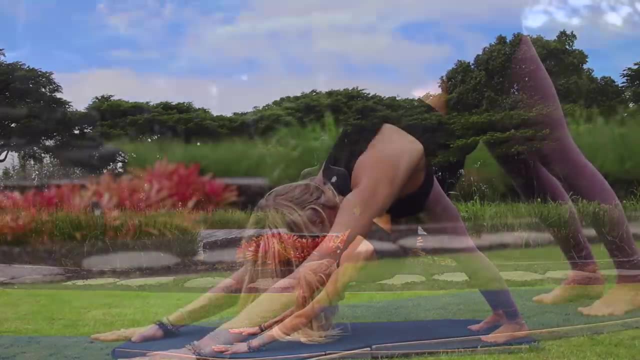 Deep breath in, Exhale, Roll yourself forward, Tuck your toes. Let's come back up into that downward facing dog. See if you can go a little bit deeper into that posture Now. if you had your knees bent the very first time? 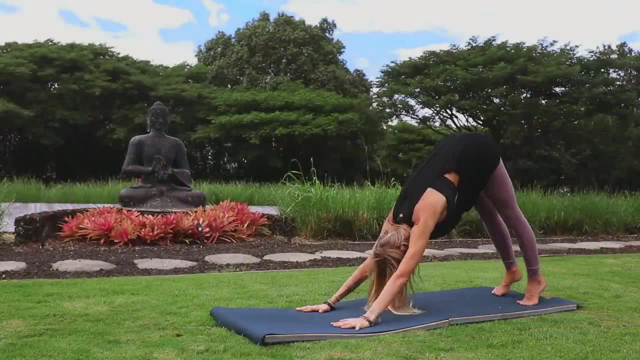 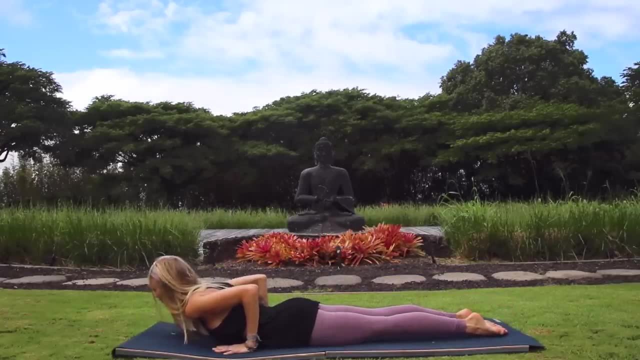 see if you can extend the knees a little bit more. Deep breath in, Exhale, come through into your plank, Chaturanga all the way down. Drop your chest to the floor From here. we're going to do an exercise to strengthen the back. 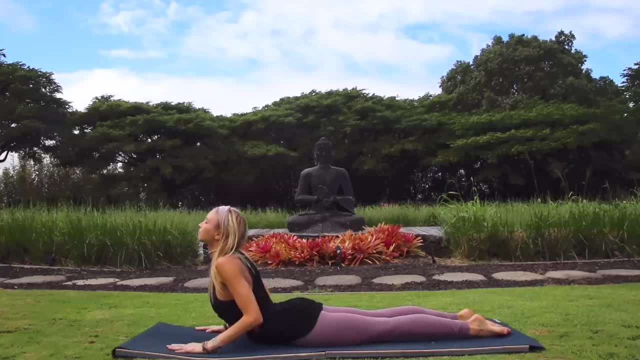 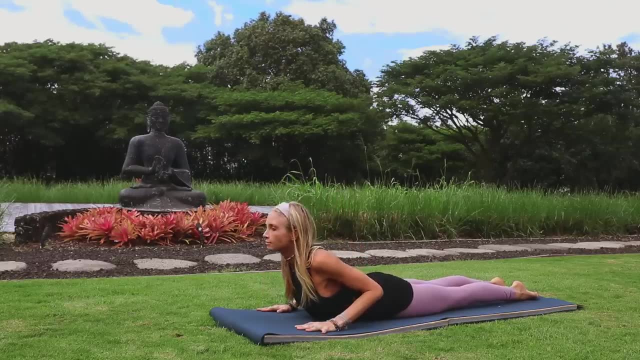 You're going to lift up, squeeze the back muscles, Keep your hands next to you, Bring it down for one Exhale, lift and hold for two seconds And down, Relax, Keep going. Let's lift up and hold. 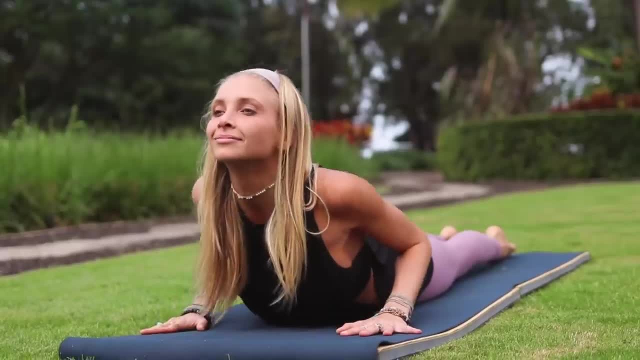 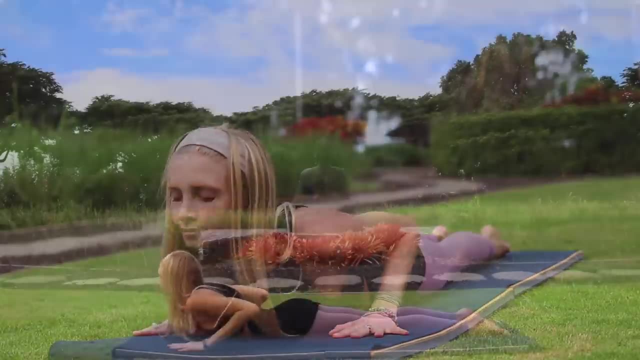 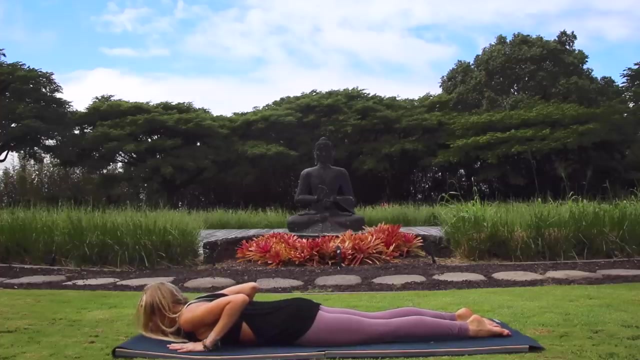 And release, Pressing the palms of your hands onto the mat next to you And release And again lift up, hold, squeeze those back muscles And release. Try not to engage your glutes here. Keep your glutes relaxed. 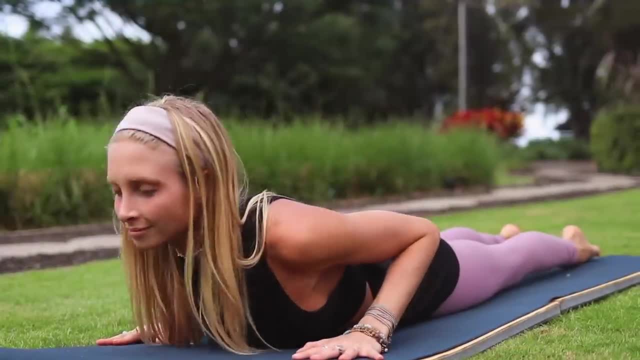 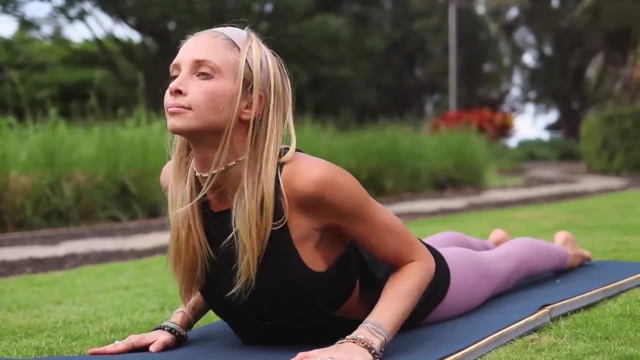 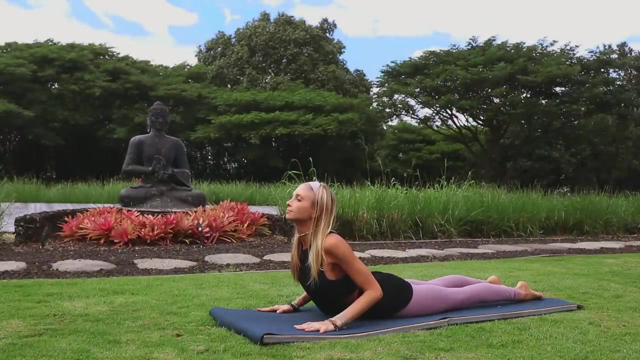 Keep your lower body relaxed. We're focusing on strengthening the glutes. We're focusing on strengthening the back muscles here. This is a great exercise for anybody that's suffering from disc herniation. This will help the disc come back into place And lower 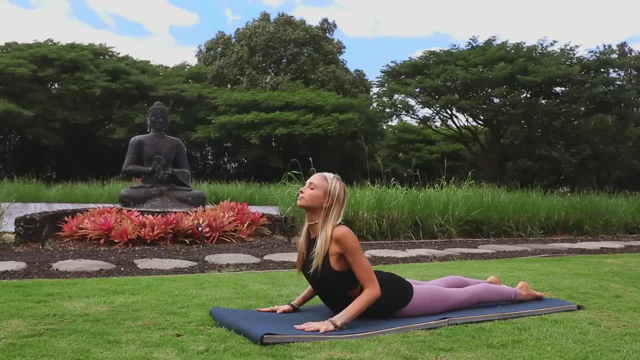 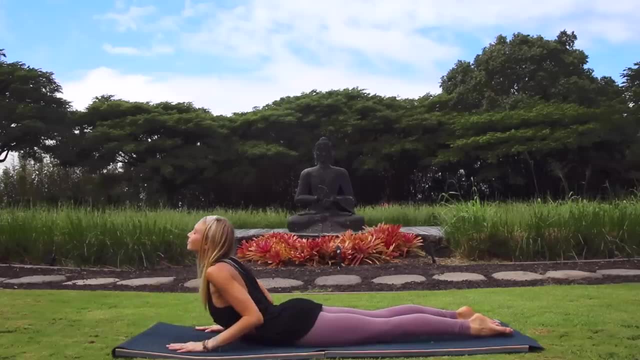 Great job. And again, lift up, squeeze And lower- Wonderful. And again, you may not be able to go all the way up, That's okay, Just do your best. Come up Even a little bit. It's the movement that counts. 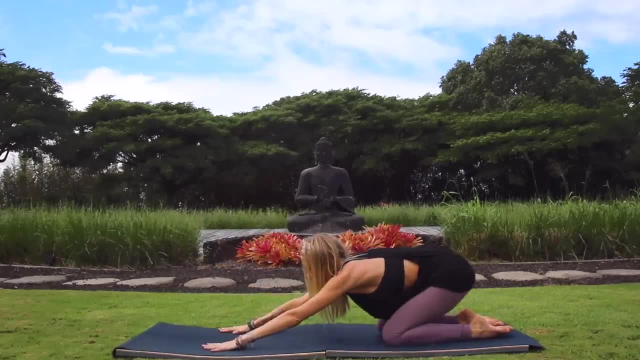 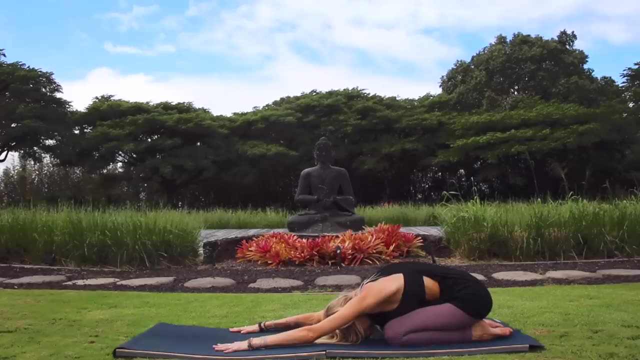 Great job. Bring yourself up to your knees And then sitting back into your child's pose, Releasing the back muscles in the opposite direction, Continuing to reach with the fingertips to the front of your mat, So you're getting into the shoulders as well. 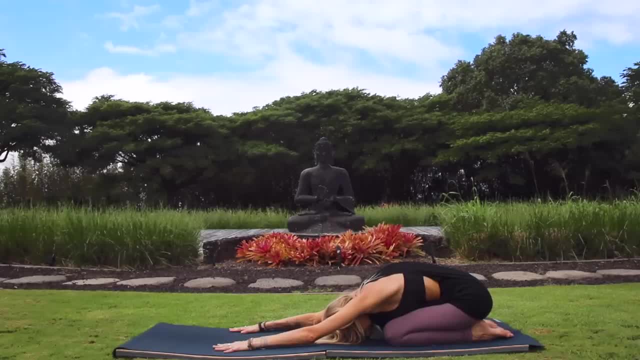 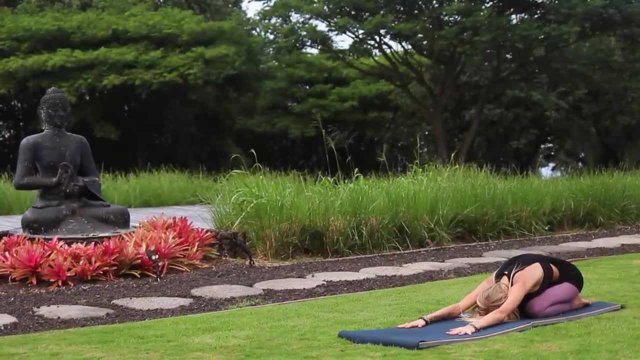 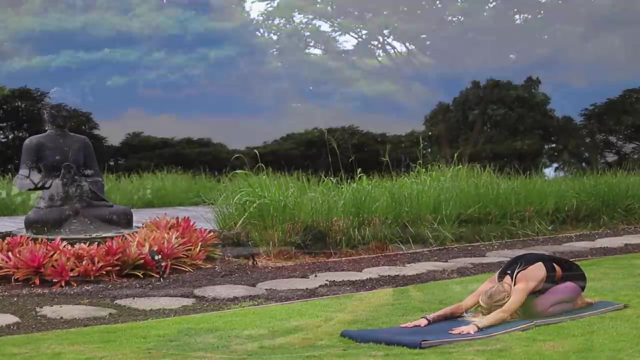 Deep breath in See how far you can release, to the heels with your glutes. Just stay present with your breath. Notice how your body's feeling right now And how you're feeling right now. How did that exercise feel on your back, on your body? 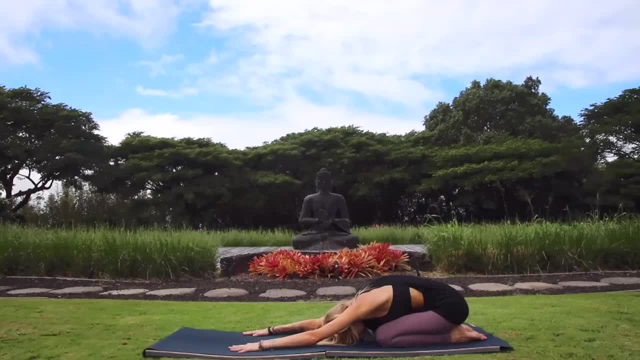 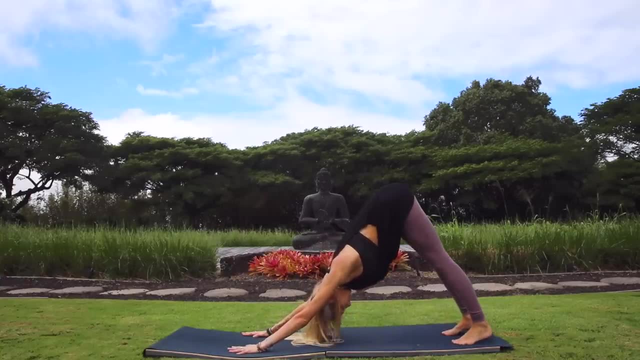 Pay attention to your body's reaction to each posture and movement. today, Come back to center, Tuck your toes And let's lift back up into that downward facing dog. Stretch those legs, Allow those heels to sink down to the floor, Take a deep breath in. 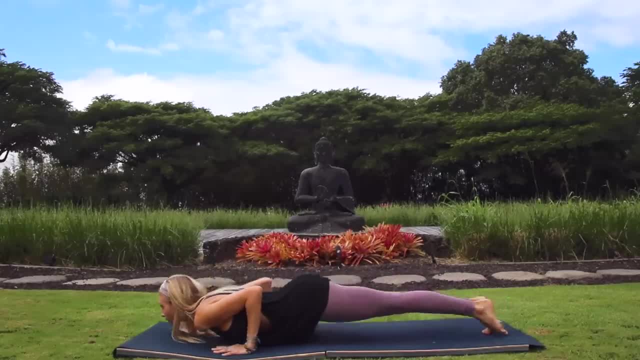 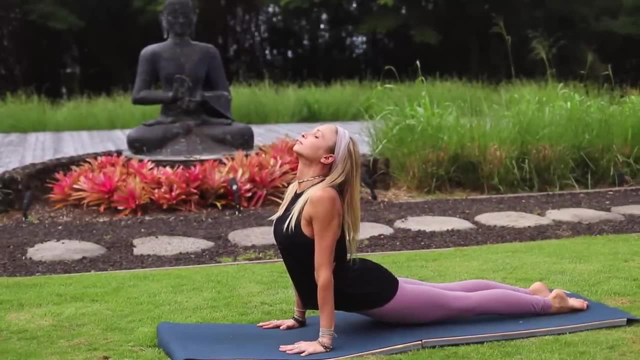 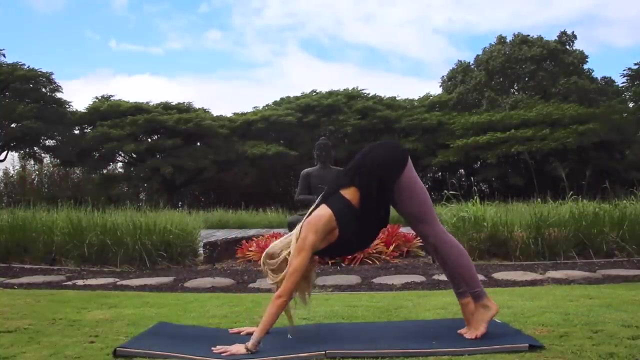 Exhale back to plank Chaturanga, This time opening into a full upward dog, if that's within your practice and you're comfortable. Otherwise, stay in the baby cobra pose, Hold Deep breath in And then exhale, bringing yourself back into that downward facing dog. 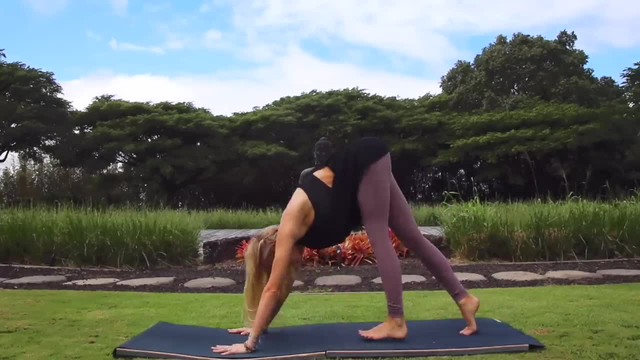 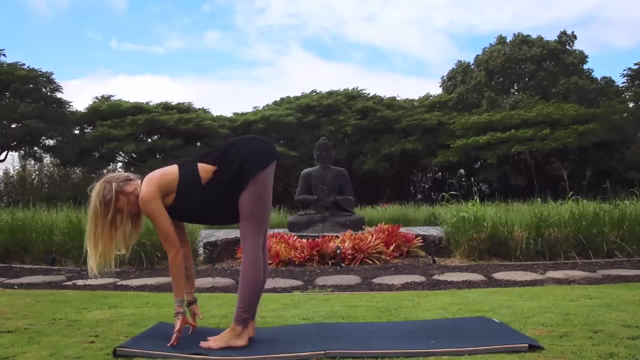 Beautiful. Let's go ahead and bend the knees and walk forward towards the very front of your mat. Take as many steps as you need Coming into a standing forward. fold. Let's inhale first. Extend through the spine And then exhale. Begin to fold forward from your hips. 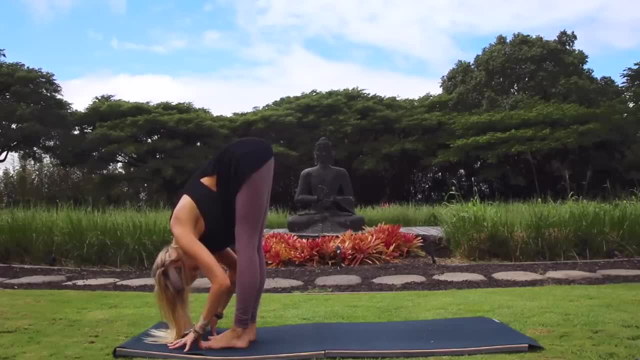 Now it's very important that you do not bend your knees. Now it's very important that you do not bend your knees. You cannot bend from the lumbar spine. You cannot bend from the lumbar spine. So if you are tight in the hamstrings, 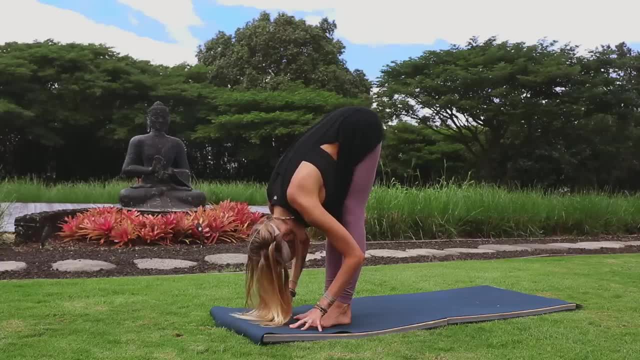 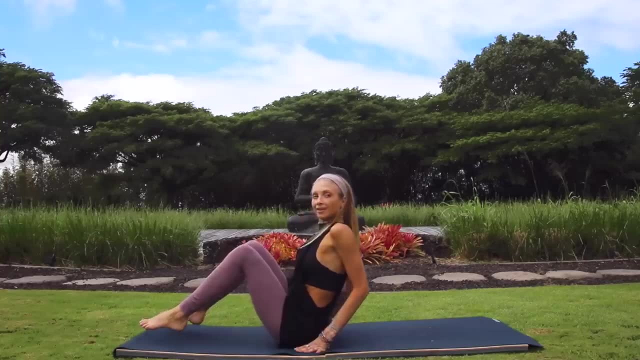 bend those knees and allow the chest to release over top of your thighs. Great job. Now, from here, let's go ahead and bend the knees And sit back over to your mat with your feet flat in front of you, Reaching the arms forward- inhale. 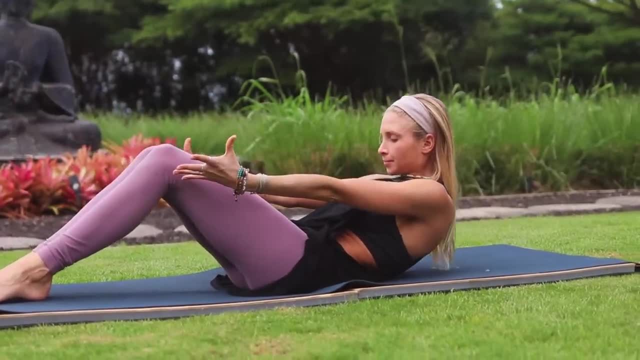 And, as you exhale, begin to release one vertebra at a time, So engaging the core muscles here, And then, once your back is on the floor, bring your knees into the chest, And also it's important to bring your knees to the chest. 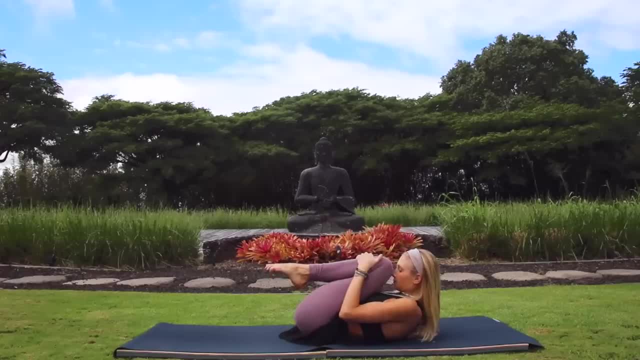 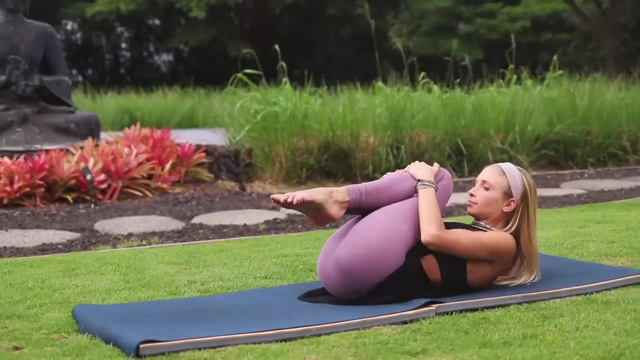 Staying in this ball position, you can keep your forehead reaching for the knees or rest your head on the floor, whatever feels comfortable for you. Let's begin to gently rock side to side- A very gentle back massage for the lumbar spine. 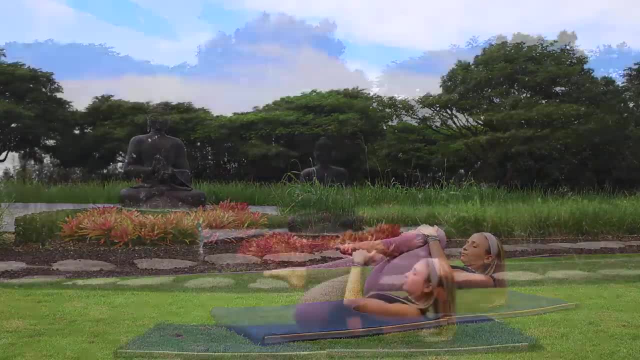 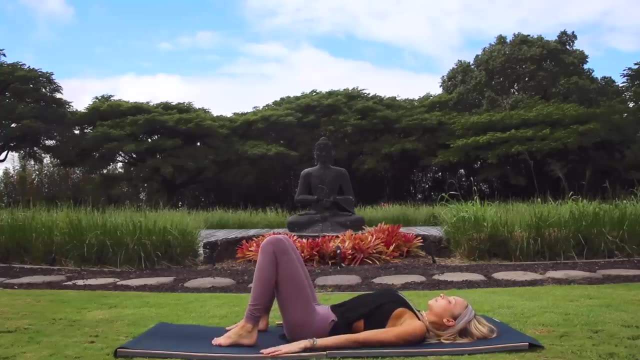 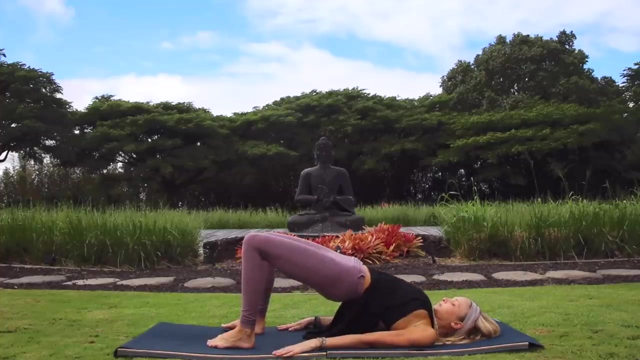 Just side to side with your breath here. Side to side, Wonderful. Drop your head to the floor, Release your feet onto the mat. From here we're going to move on to a next exercise, again to help strengthen the back. You're going to lift your pelvis all the way up, squeezing the glutes here. 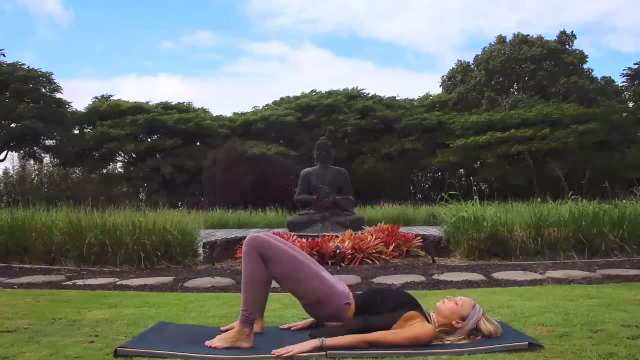 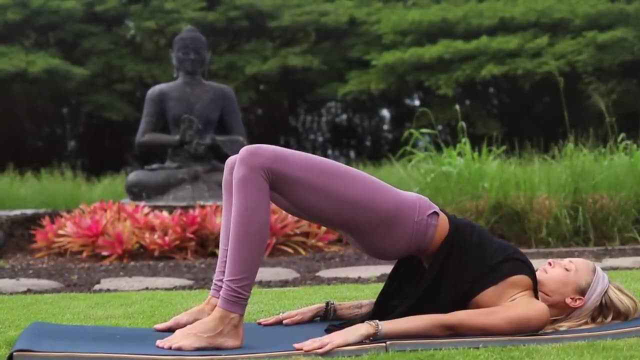 Baby bridge position And then slowly releasing through each vertebra of your spine. So when you lift, first start with the tailbone- lower back, mid-back Lifts up, Hold and squeeze And then, as you exhale, reverse it, Start from the middle. 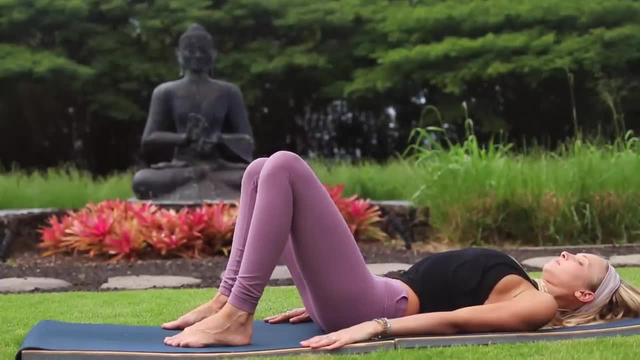 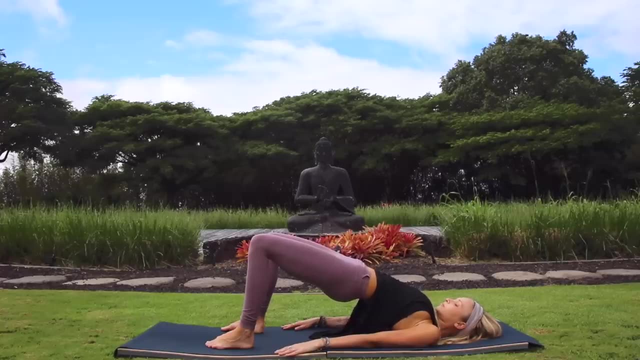 Back, lower back and tailbone to the ground Again, lifting up, Engaging your glute muscles here, Squeeze and lift those hips up towards the sky And slow with control. So this particular exercise is all about finding that control in the movement. 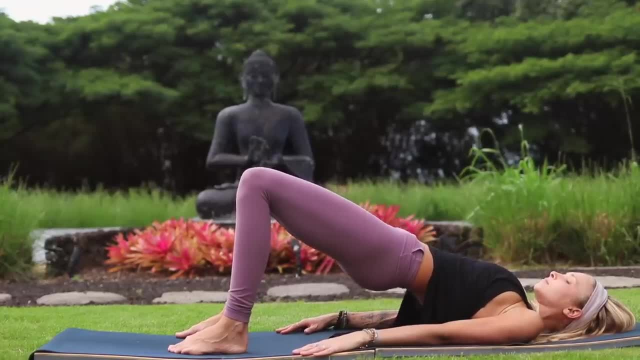 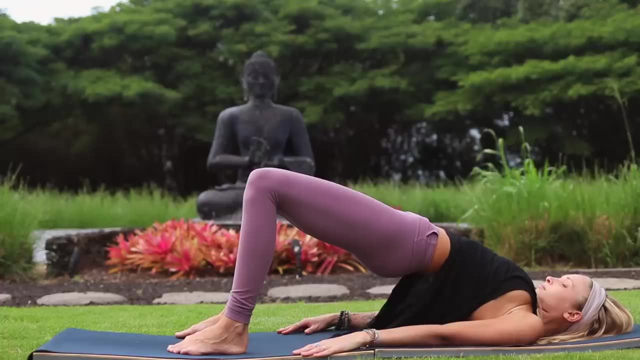 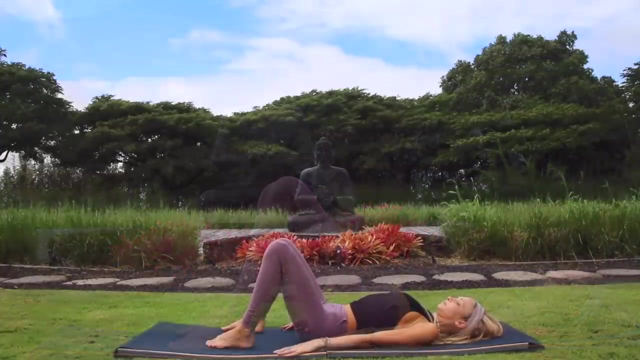 Do not rush, Do not go too fast, Just slow and steady. Again, lift from the tailbone, Lift up, Squeezing the glutes, Lift as high as you comfortably can And then release through each vertebra of your spine And again tilt, Lift, Squeeze. 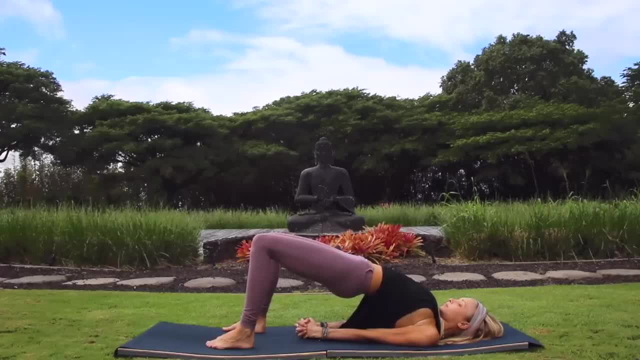 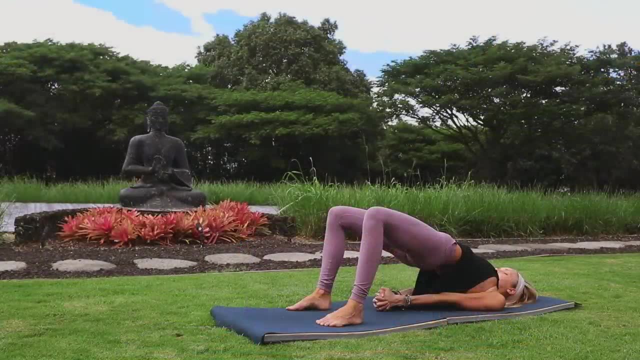 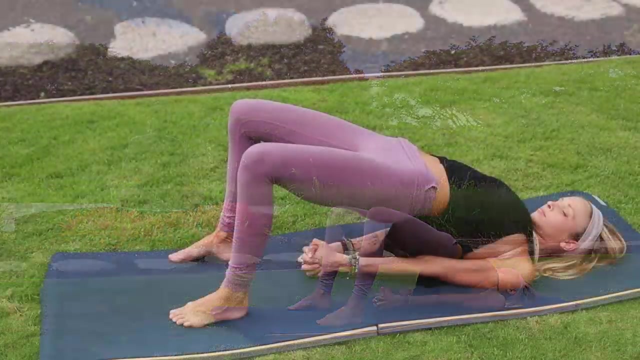 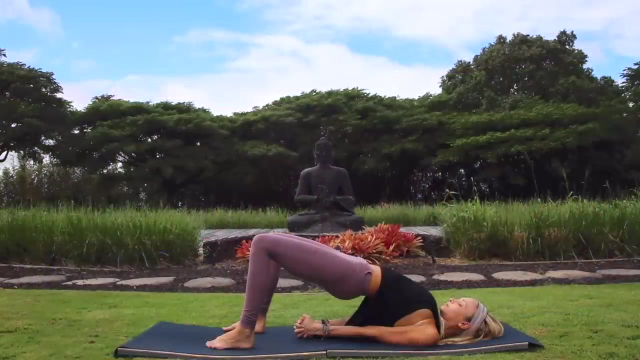 Stay there, interlacing the fingers and holding that bridge position a little bit longer now, Squeezing the glutes, Breathing deeply here, Staying with your breath. Do not allow your hips to drop. So the engagement of your glutes. 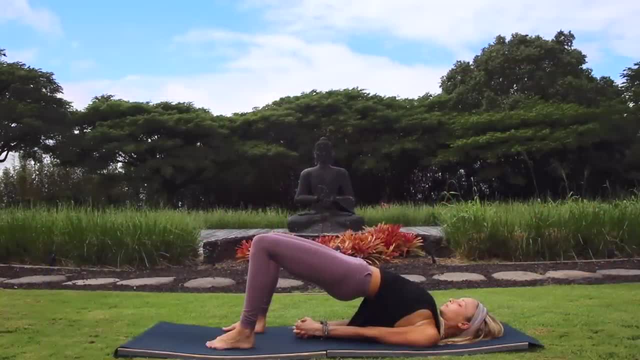 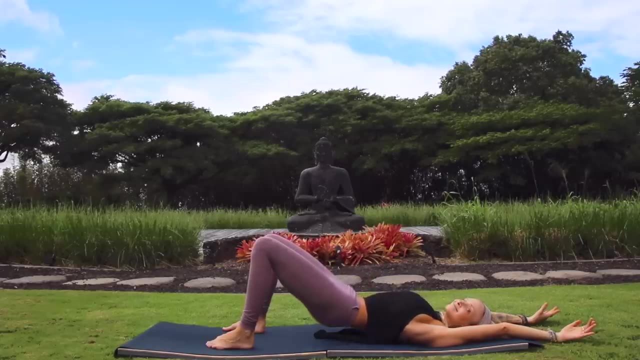 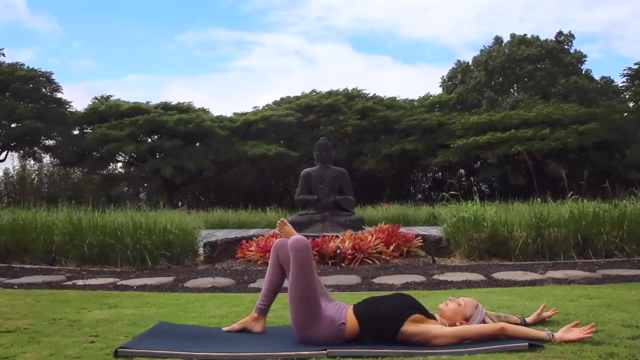 your lower body is extremely important here. Lift a little bit higher And then reach the arms over your head And then slowly begin to release the spine through each vertebra of your spine. Beautiful job. Once you release your back, you're going to take your left leg and place the ankle. 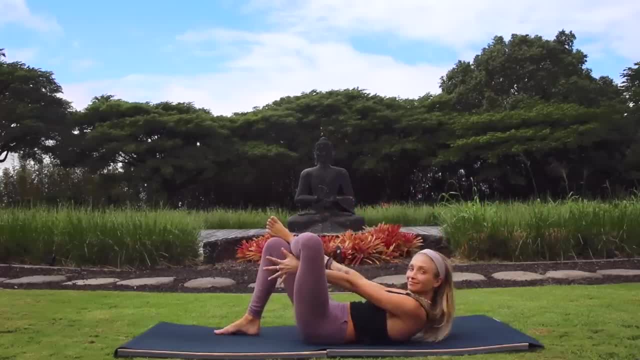 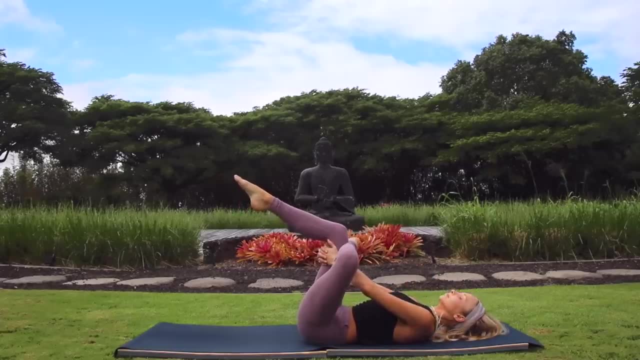 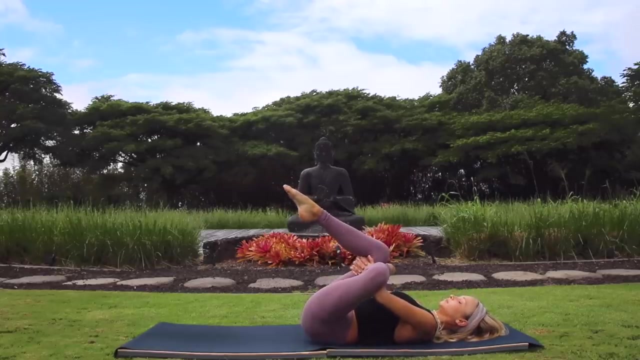 over top of your right knee. Bring the arms forward. Now take your left arm through the legs and then attach both of your fingers behind your right leg. From here, drop your head to the floor and begin to pull the right knee into the chest. This is called your Reclined Pigeon Pose. Now, if you'd like to go, 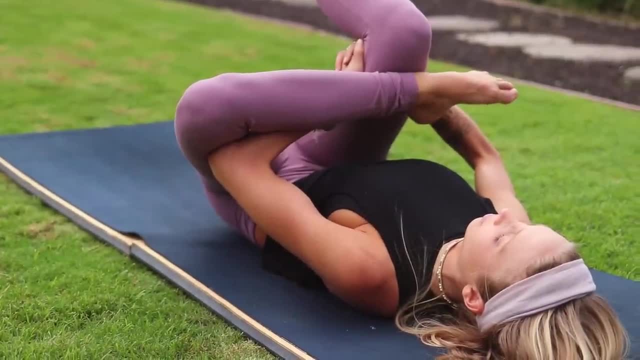 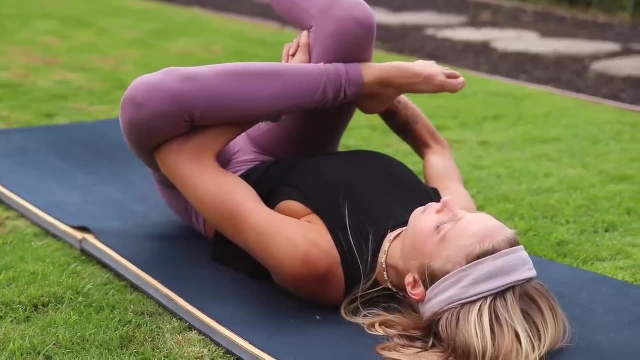 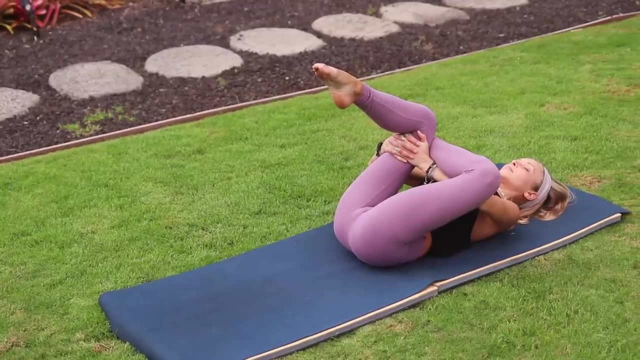 a little bit deeper. you can use your left elbow and push that left knee away from you as you pull the right knee towards you. What we're doing here is going a little bit deeper into that glute muscle, into the piriformis. If you do suffer from any sciatica pain, this is a wonderful posture for. 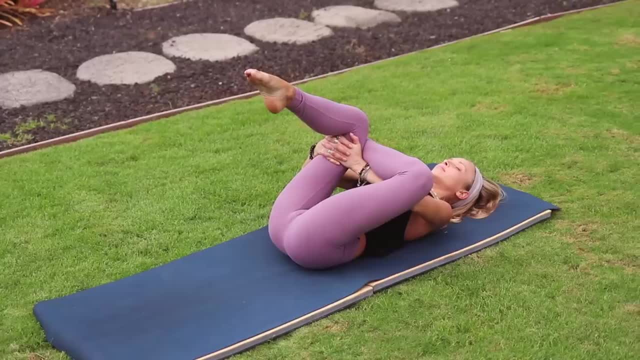 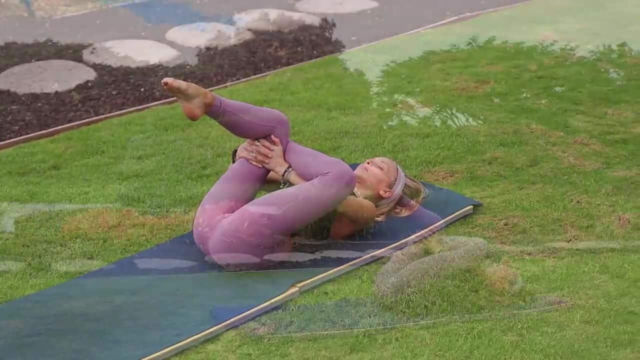 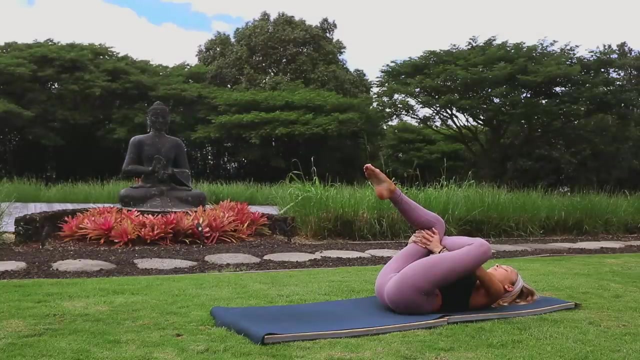 you to do every single day to help loosen that area where that nerve might be pinched. So breathe deeply And with each exhalation see if you can pull that right knee closer to the chest And at the same time push the left knee more further away from your body with your 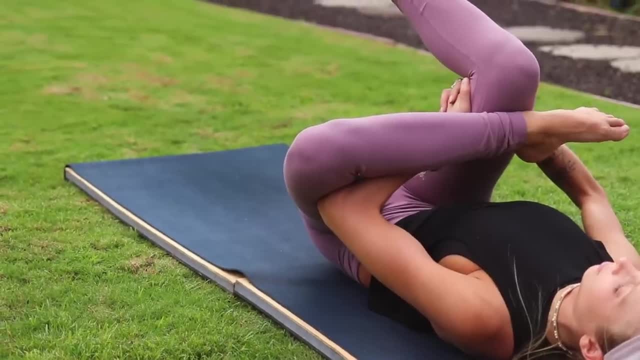 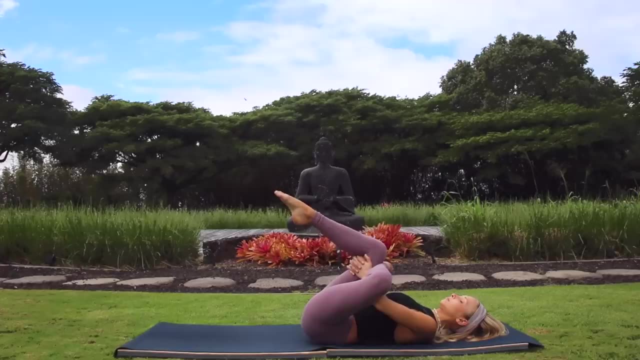 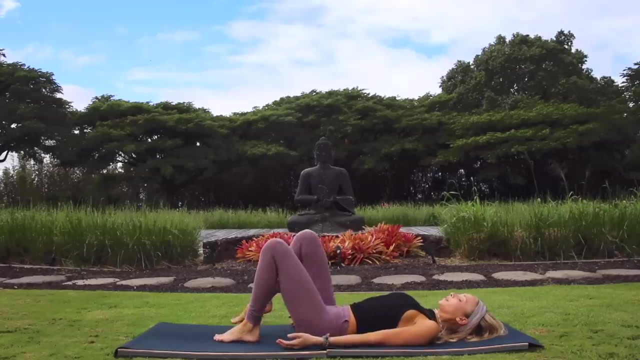 left elbow. Notice how your body is responding to this particular posture. Great job. from here, We're going to extend both legs and then drop your feet onto the mat And we're going to go right to the other side. So now, right ankle over top of your left knee, Bring that leg up. 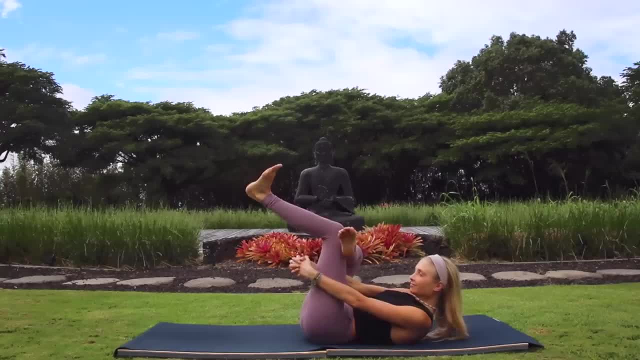 Right arm is going to come through between the legs. Wrap those fingers around, Place the fingers behind your left knee And then bring those fingers together And then bring that leg up And then bring those fingers together And then bring those fingers together And then bring those. 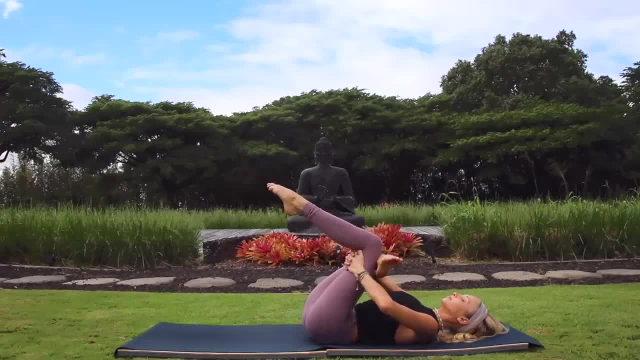 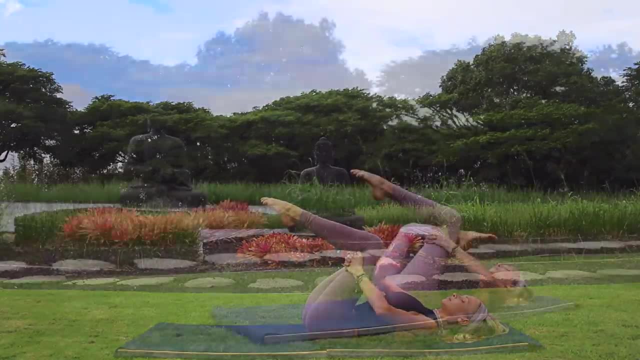 leg. Begin to pull the left leg towards your body. Now use your right elbow to push the right knee away from your body. So it's a pull and a push kind of movement, here Done at the same time, so you're getting that maximum stretch into. 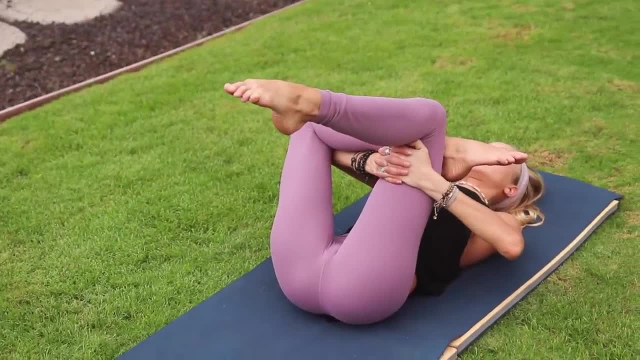 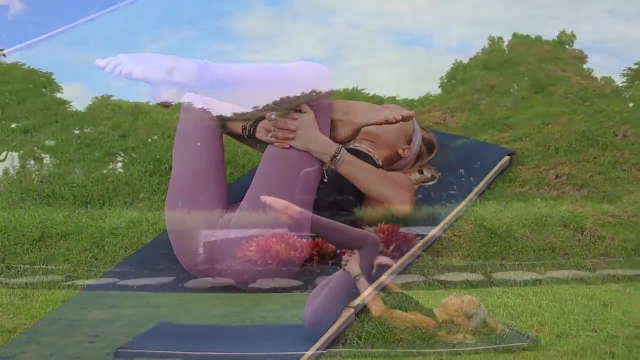 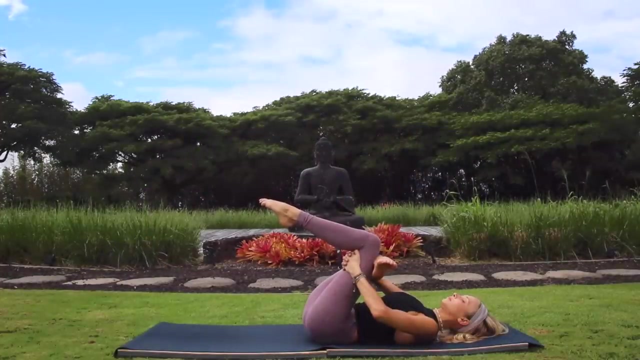 the right glute muscle Breathing deeply and hold, Making sure that your neck is relaxed. You're not tensing up your upper body. Head is on the floor. Feel free to close your eyes. Go inward. Pay attention to how your body is feeling. 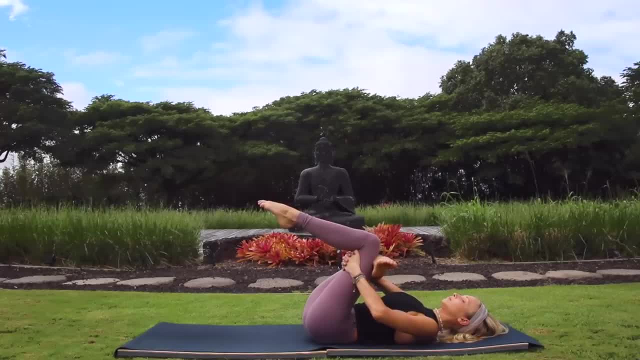 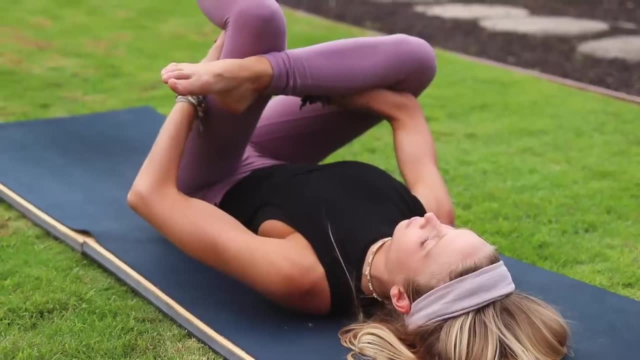 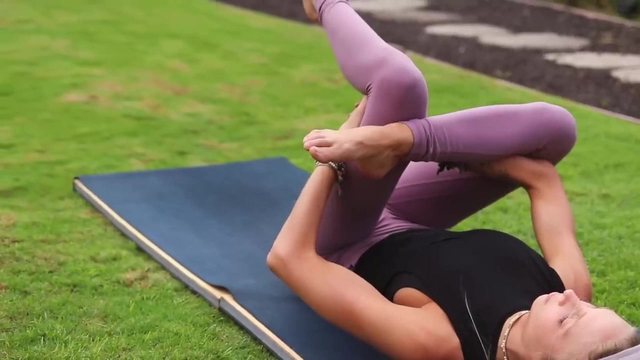 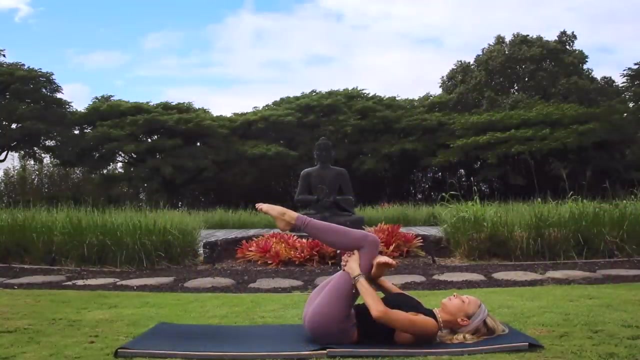 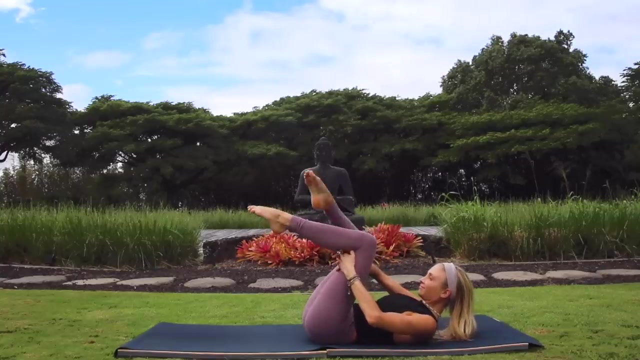 right now. What kind of thoughts are entering your mind? If they are negative thoughts, allow yourself to exhale that energy out. In order for our bodies to heal, we must take care of ourselves. Let's take one more deep breath in Exhale, releasing the legs. Extend both. 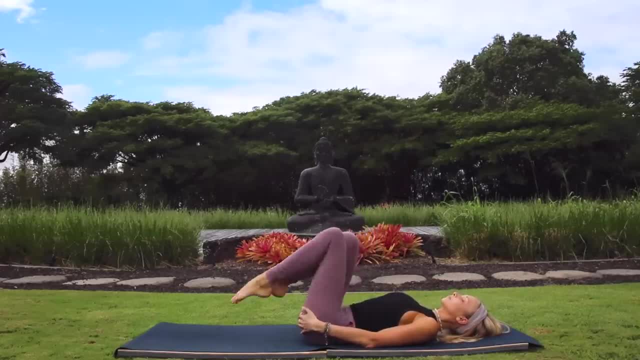 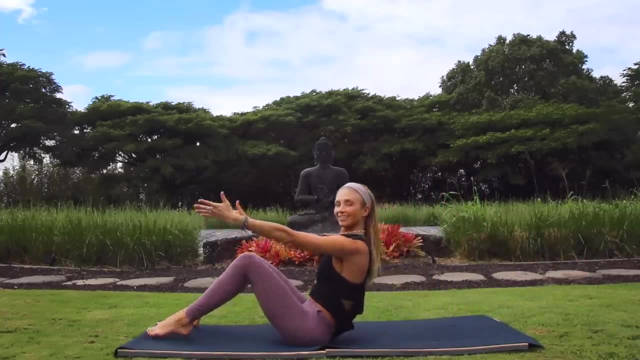 legs up and then, from here, drop your feet to the floor, Reach the arms over your head, rolling yourself up. Now use the strength of your core muscles, Come up to seated, Cross your feet in front of you and transition back into that plank. 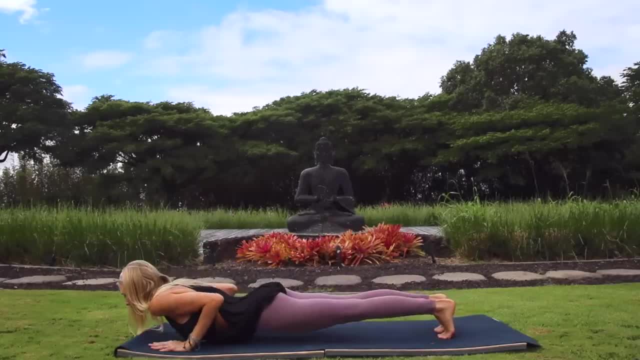 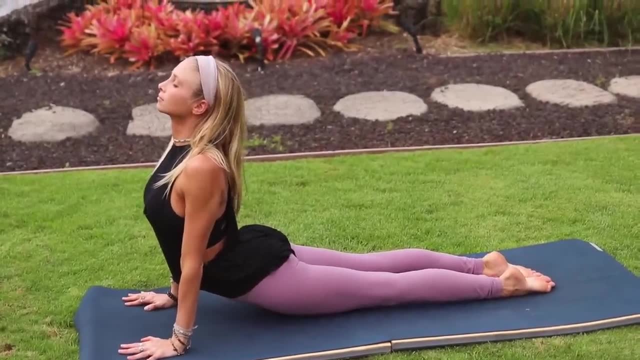 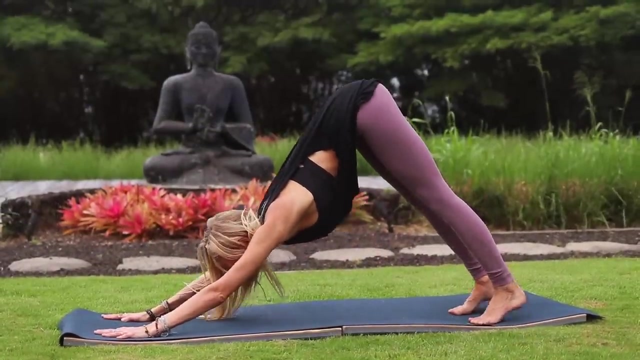 position: Inhale, Exhale. let's go down and through that chaturanga Upward facing dog or baby cobra, whatever you're comfortable with- Hold and then exhale, releasing back into that downward facing dog Inhale. As you exhale, begin to walk forward with. 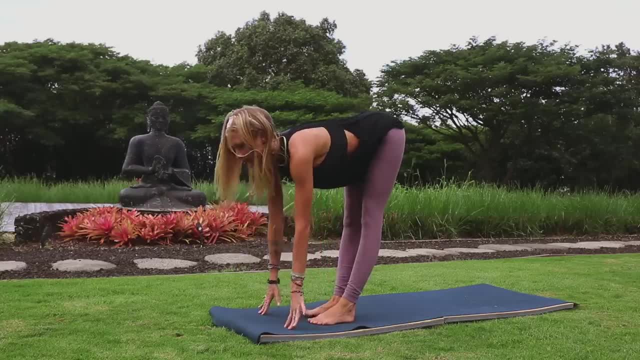 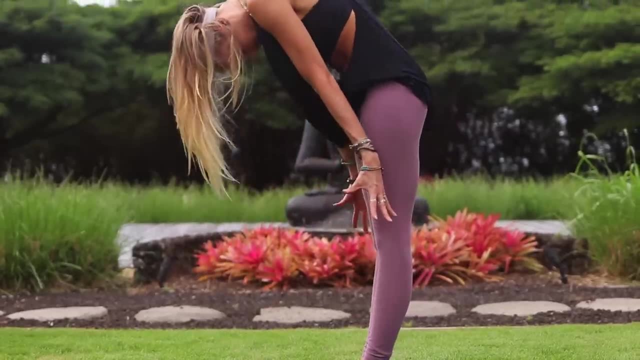 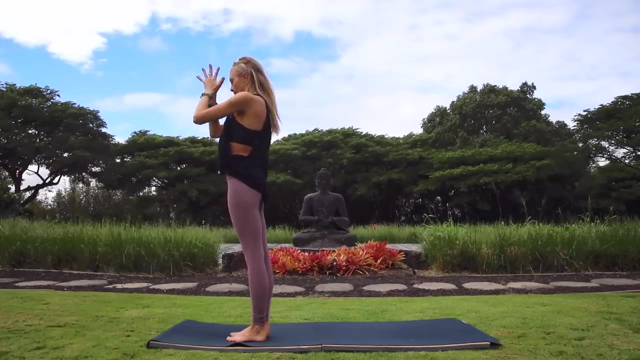 your feet to the front of your mat, again, Feet together and slowly coming up halfway. Exhale, release into the forward fold. Inhale, rolling yourself up to standing now, reaching both arms up to the sky, palms together. Exhale, bring your hands to your heart. Just find that center. 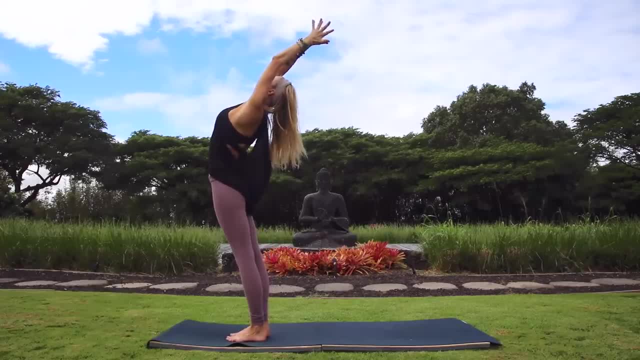 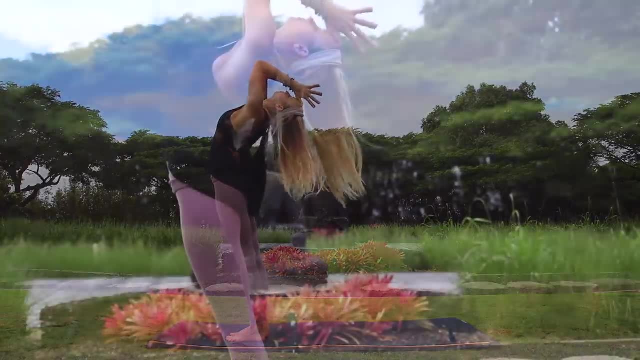 Inhale again, reaching both arms up. Exhale a gentle backbend if you're comfortable. Otherwise stay upright, Hold it there and breathe. Exhale, releasing yourself forward into that forward fold. Inhale halfway lengthen. 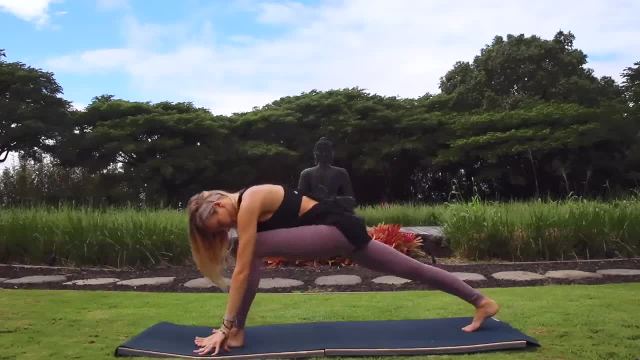 Exhale release into the upward fold. Inhale half way lengthen. Exhale release into the upward fold. Inhale half way lengthen. Inhale half way lengthen and then exhale. you're going to step your right leg all the way back. 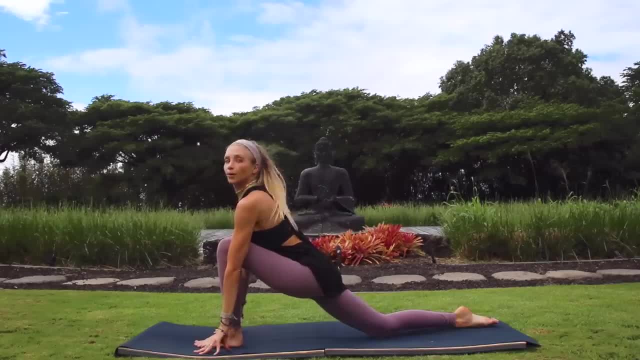 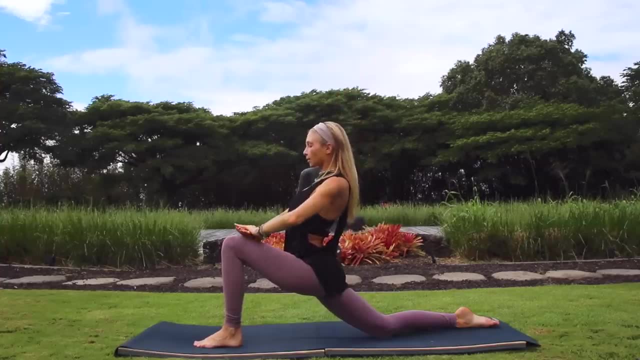 you're going to drop the right knee to the floor and once you're ready, you're going to reach both arms up towards the sky into that low lunge. now bring your hands over top of that left knee and lift your hips up a little bit higher if you need to, but i want you to. 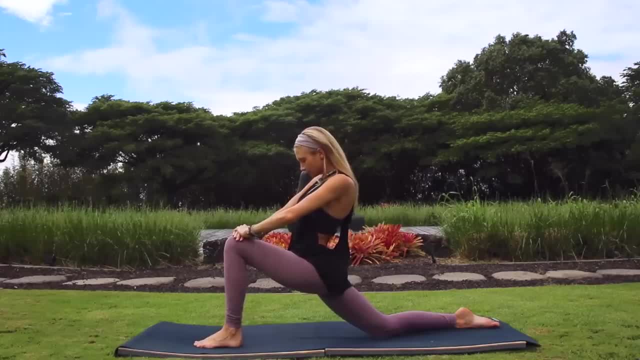 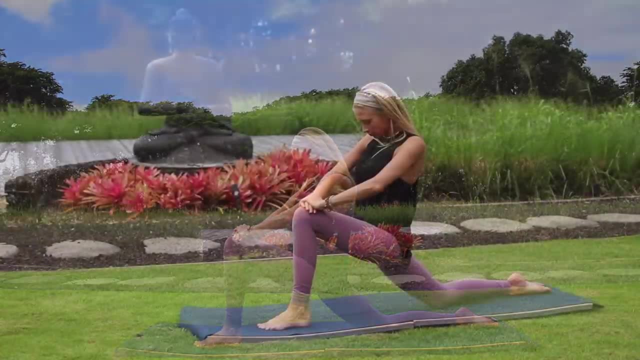 really find that position where you're targeting the psoas muscle, your hip flexor. so for everybody it's going to be slightly different. some might need to come down lower with the hips, others might need to come up higher. so stay here and just play with it. a. 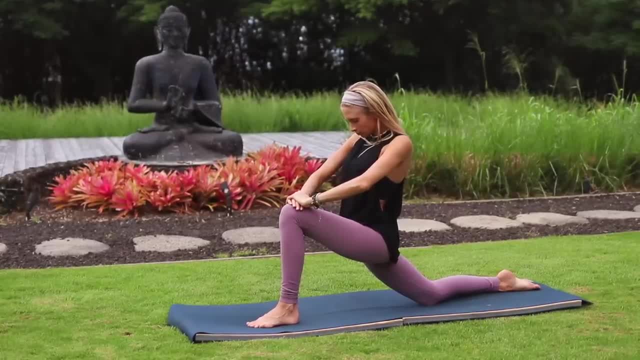 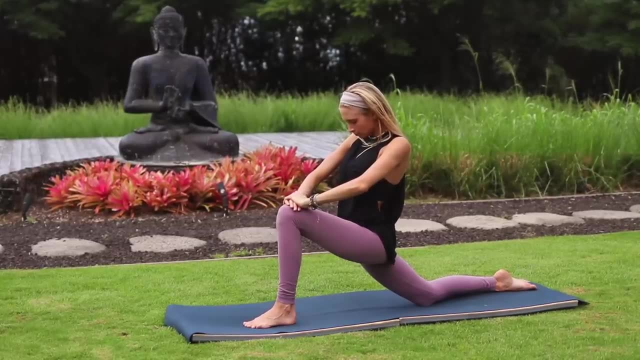 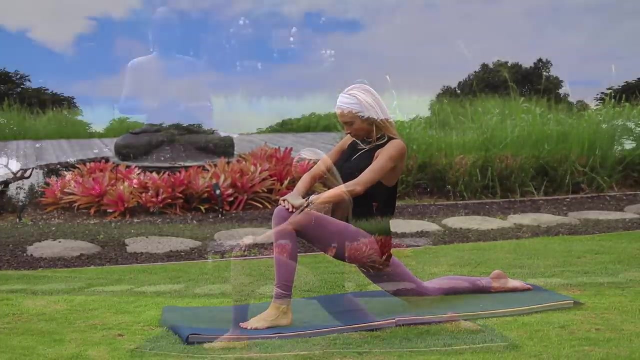 little bit, finding that particular posture that suits you best. keep pressing into that front knee with both hands, tuck the chin down towards the chest, just breathing deeply. it's really incredible in the way that our muscles are connected to each other, so even if you might be experiencing low, 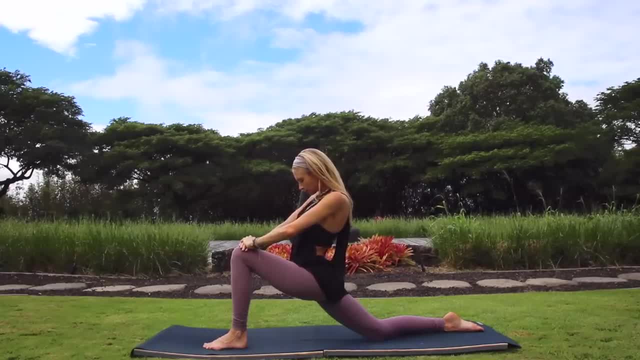 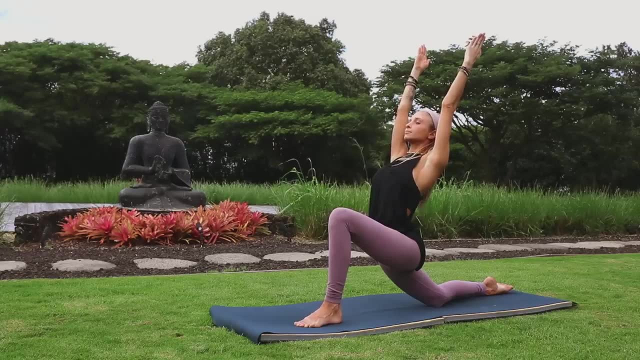 back pain, you're going to be able to feel that pain. the origin of that particular injury might actually come from your hip flexor. let's inhale, lift those arms up to the sky again and then, as you exhale, drop your hands to the floor. you can use blocks here if you need to. 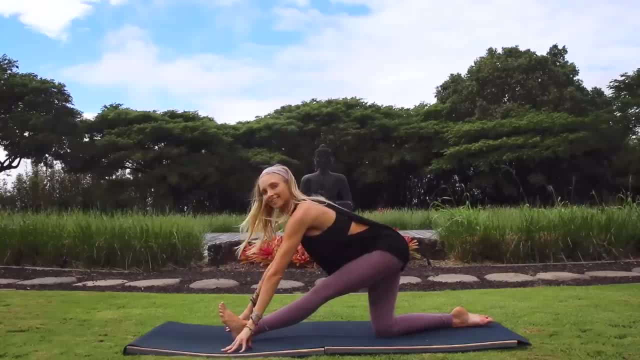 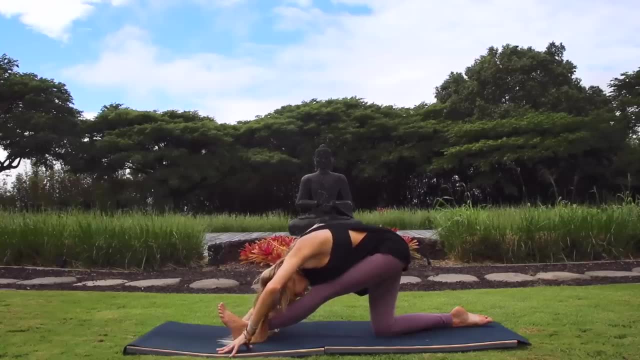 or any other props pushing your hips back now, flexing your foot and then making sure your hips are square. so pull that left hip back, push the right hip forward and release yourself over top of your leg. have split posture this time. now we're going deeper into. 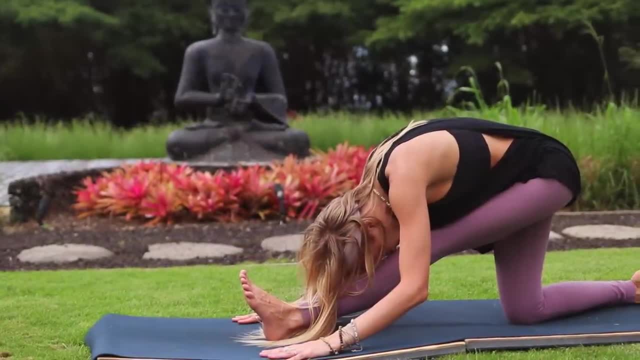 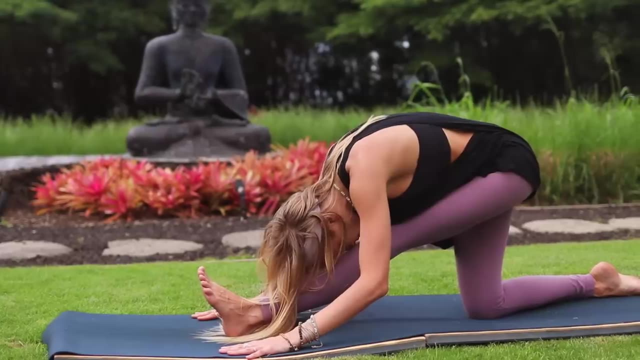 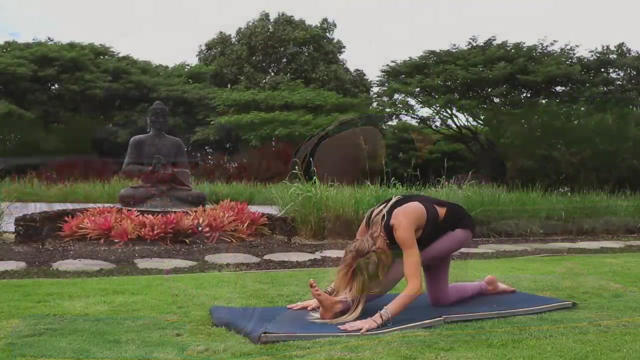 the hamstring, keeping that front foot flexed, with each exhalation feeling not only a release through the hamstring but also through the calf muscle all the way down to the heel. just breathe and let go wherever you are here, whether your forehead is touching your knee or you're upright. 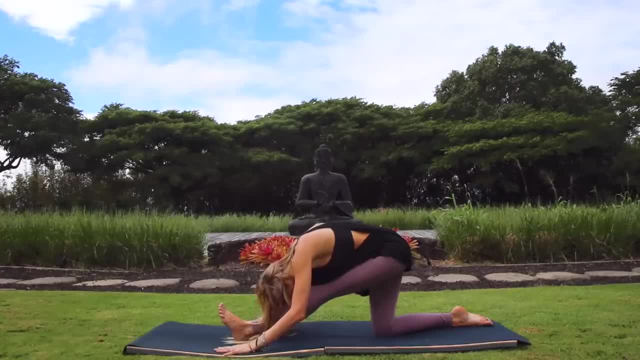 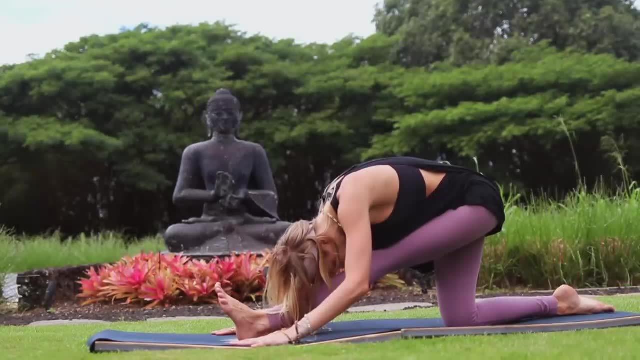 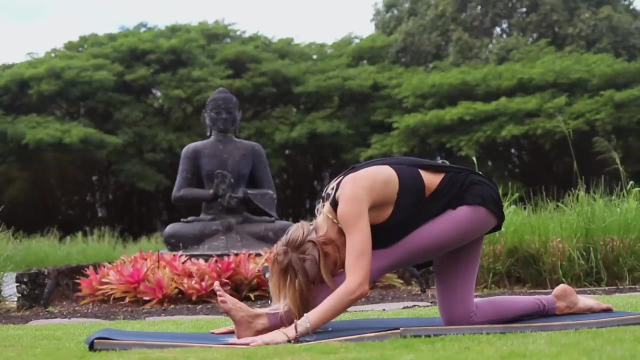 being patient with your body. never let go of any of the muscles in your body, knowing that it will take time for your body to release deeper into this posture. so just stay wherever you are and focus on relaxing into this pose with each exhalation: deep breath in, exhale out. 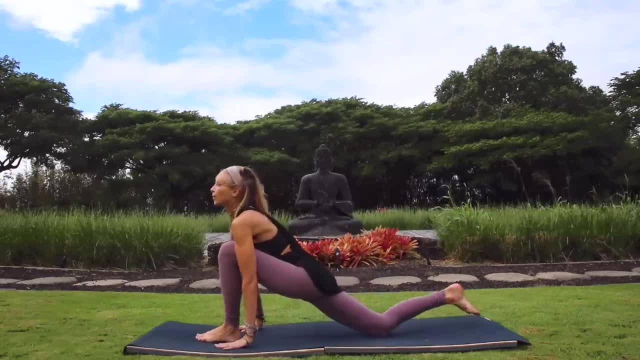 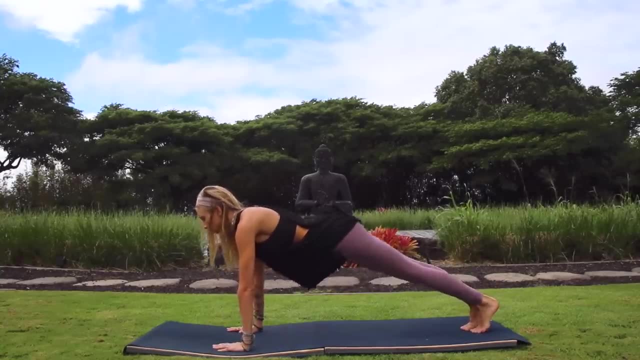 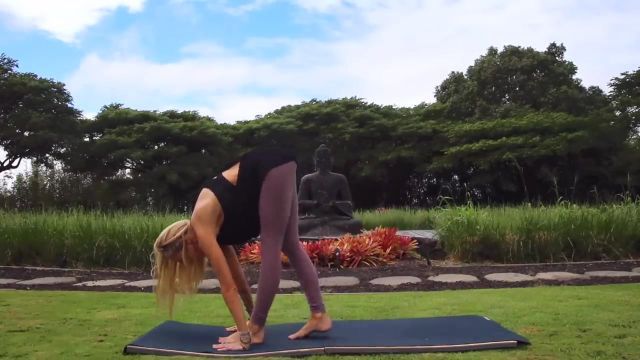 beautiful. now slowly come back to center, bringing your hips forward, tuck your back toes and lift your back knee off the floor and then stepping back into that plank and pushing your hips back into the downward facing dog deep breath in exhale. walk your feet forward towards. 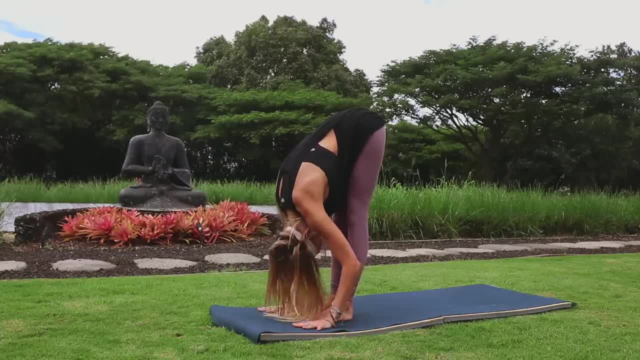 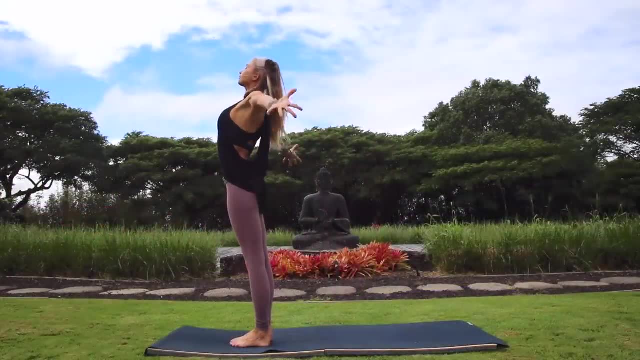 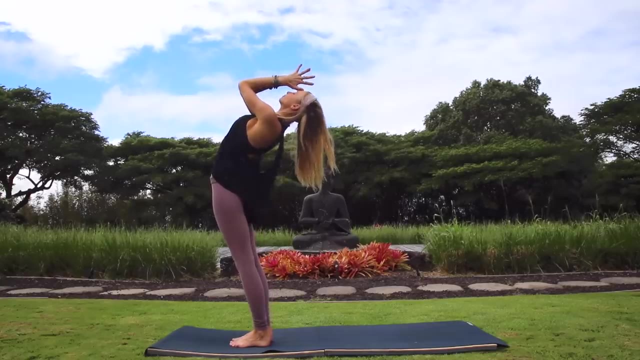 the front of your mat. inhale from here we're going to come up halfway. exhale forward, fold. inhale rolling yourself up to standing, reaching both arms up to the sky, and exhale hands to heart or chest to chest- a heart or a gentle back release. 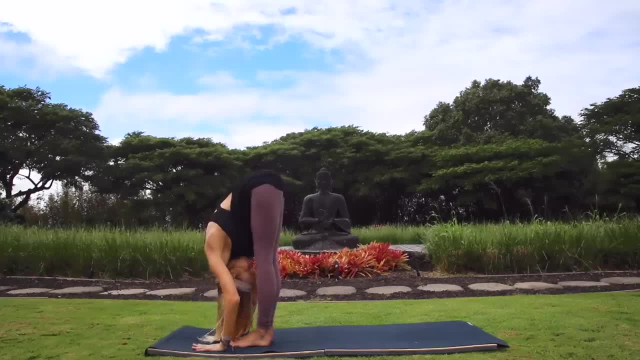 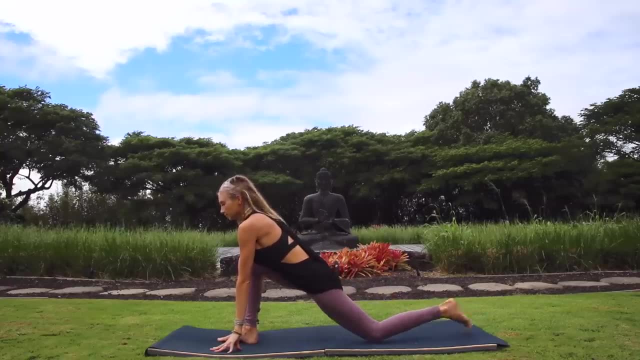 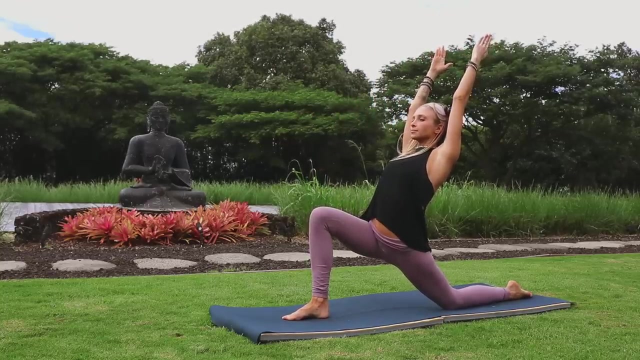 coming back to center and releasing forward into that forward fold, inhale, halfway exhale, step your left foot back and then, from here, drop your back knee to the floor, reaching both arms up to the sky into that low lunge. from here, another inhale and as you exhale, we're going to release your hands. 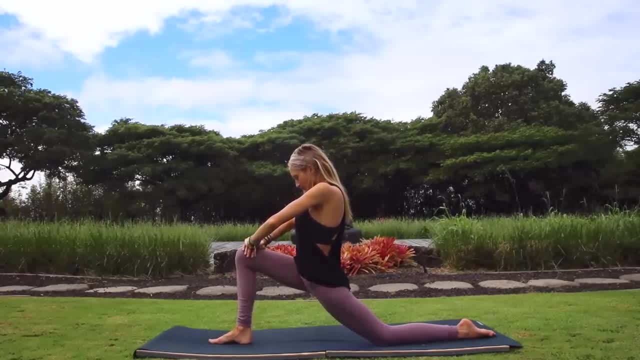 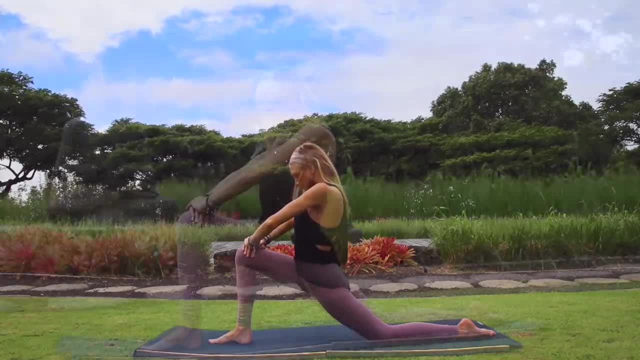 over to that front knee. you're going to push into that front knee as you bring your chin to the chest and now the positioning of your hips is going to vary. you may want to come forward with your hips, making sure you're not passing the front toes with your knee, or you might want to come back a little. 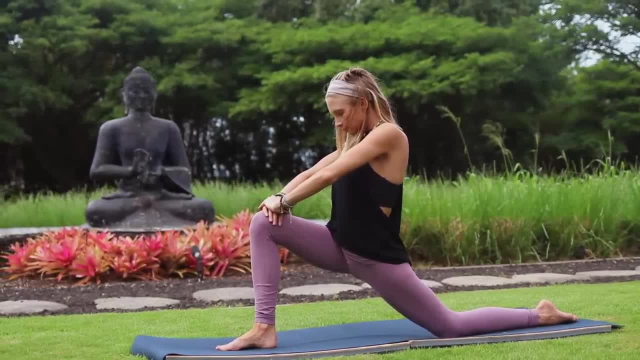 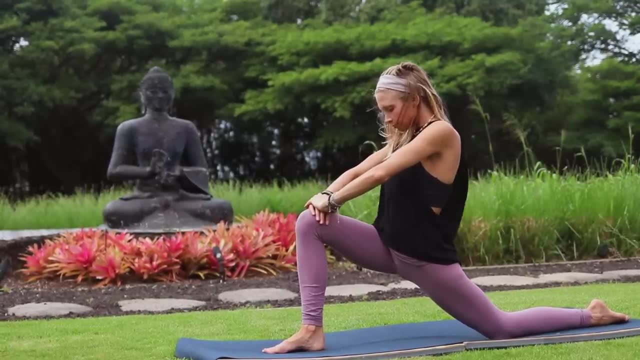 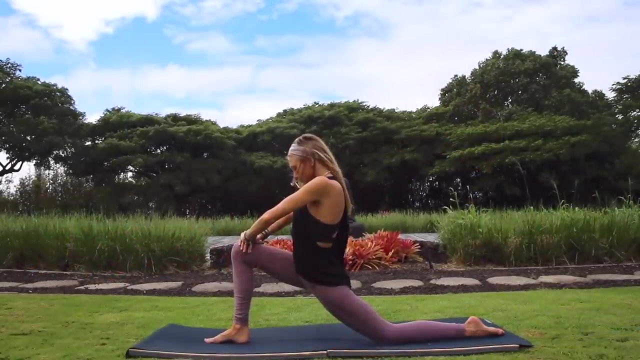 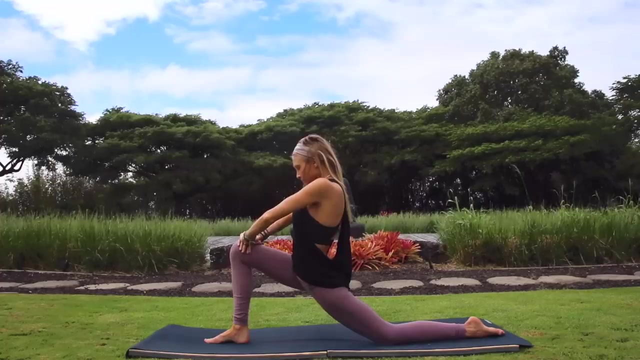 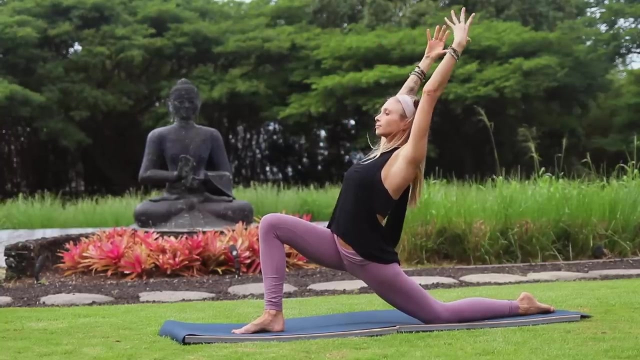 bit being more of an upright position. whatever it is, play with it and then find that particular posture, that particular point where you feel the maximum release in that hip flexor. stay here and just breathe for a moment. so beautiful. now let's reach both arms up to the sky. 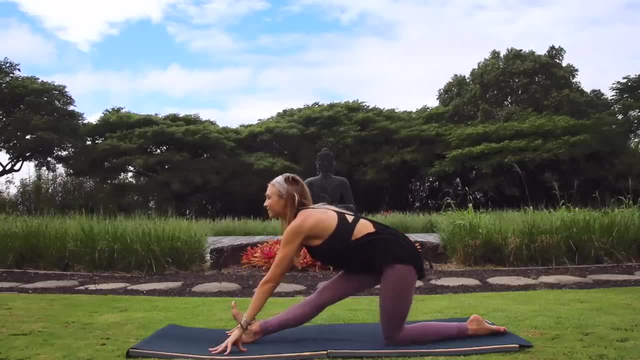 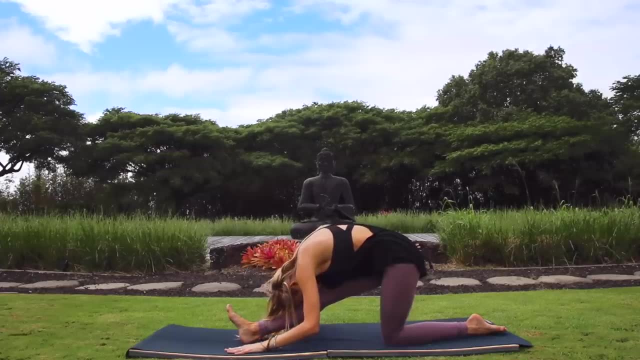 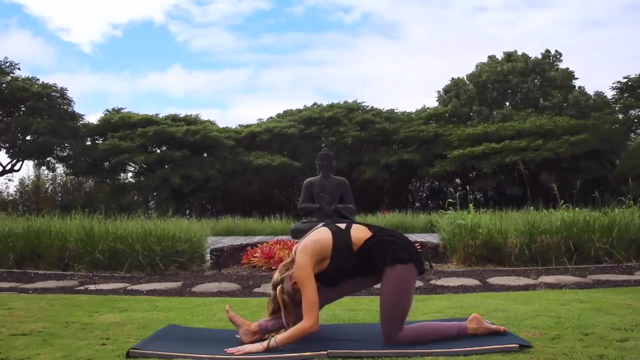 releasing your hands to the front, pushing your weight back, flexing your front foot, and then, once you're ready, begin to release your forehead to your knee into that half spin split, pulling the right hip back and pushing the left hip forward, flexing those toes towards your head, really feeling that release through the. 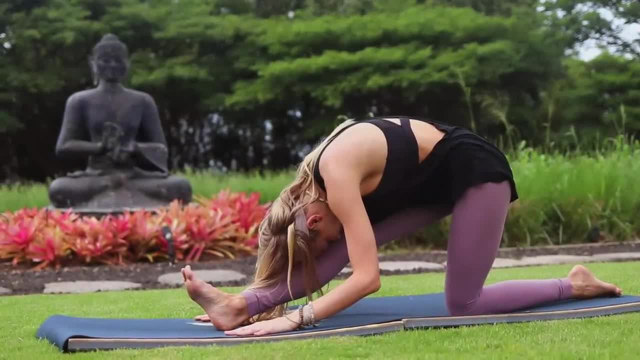 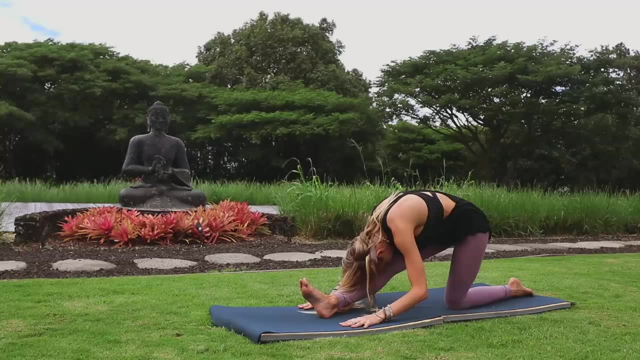 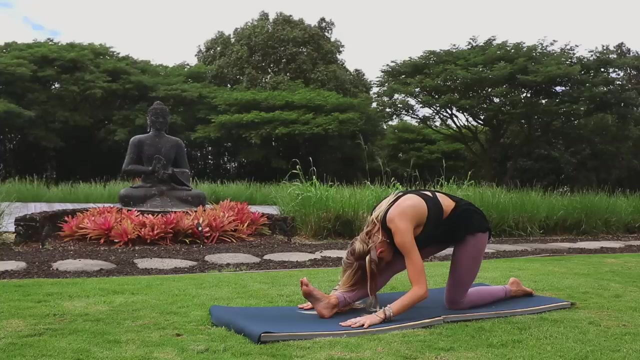 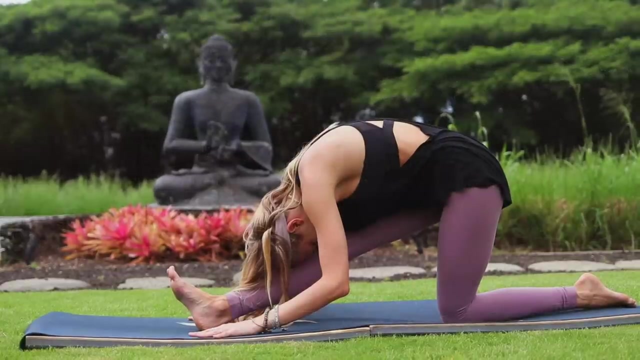 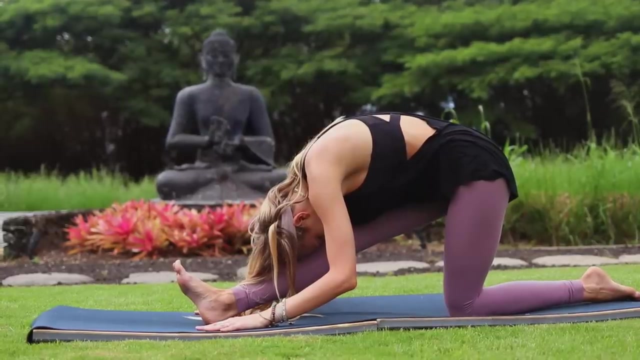 entire back of your leg, breathing deeply here, letting go. visualization is a wonderful technique that you can do while you hold these postures, visualizing tension or even pain melting away out of your body, away from you, exhaling any negativity, any frustration you may feel, especially if you're recovering from an injury. 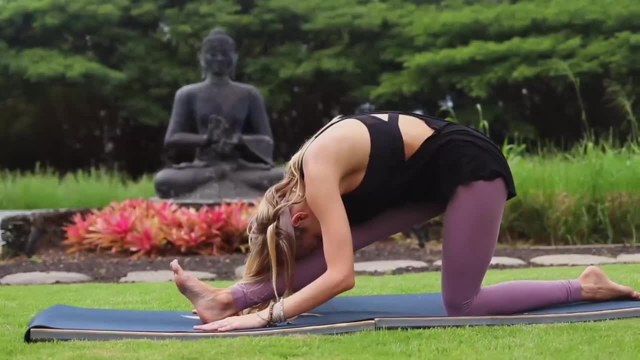 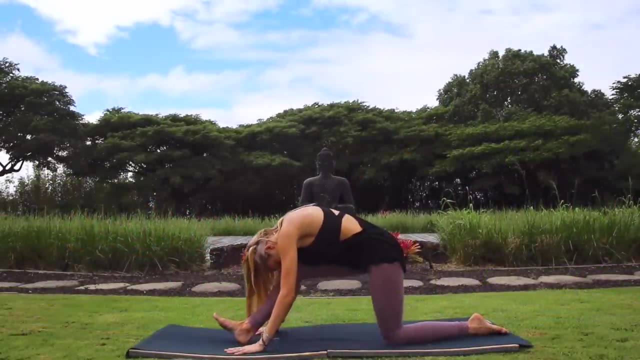 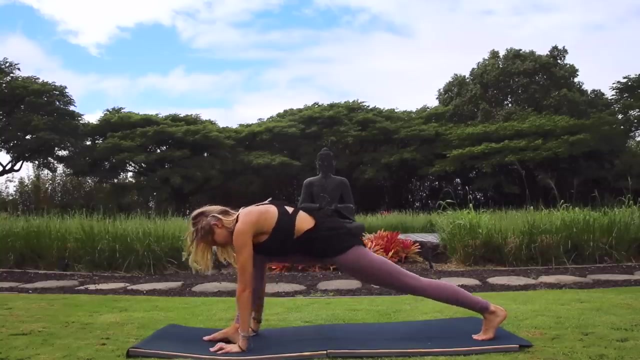 it's very normal to feel frustrated, but just know, what you're doing right now is exactly what your body needs to heal itself and to get back to normal. come back to the center with your hips, tuck your toes, lift your back knee off the mat and let's step back into 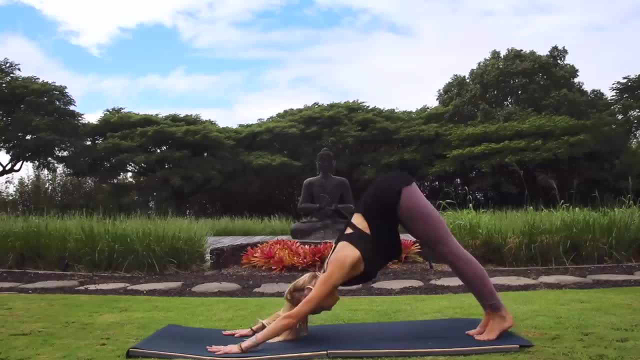 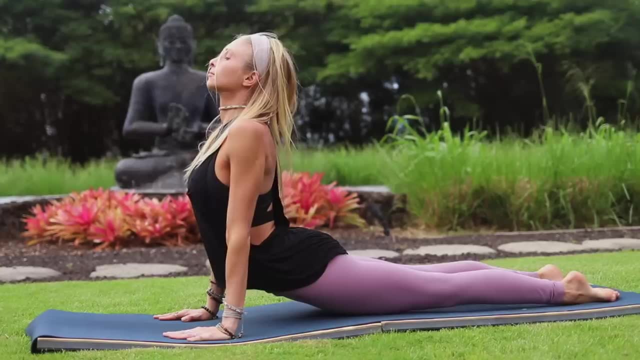 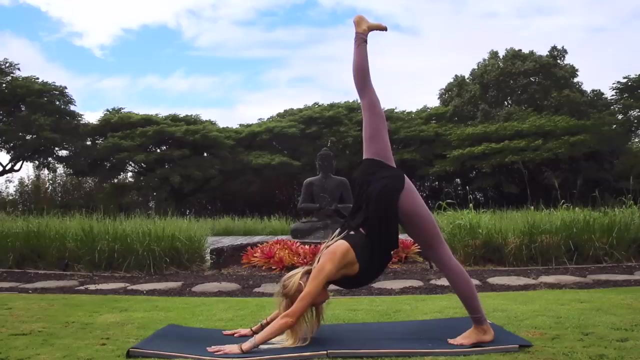 that downward facing dog. great job. deep breath in, exhale, come through to plank chaturanga, baby cobra or a full upward dog, if you're comfortable, and back into that downward facing dog, inhale, reach the right leg up to the sky, bend the knee. at this time you're going to bring your right. 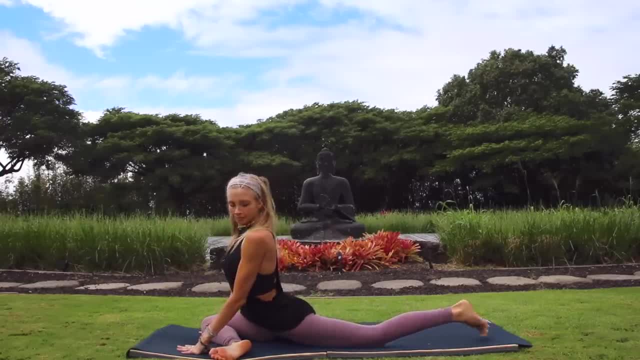 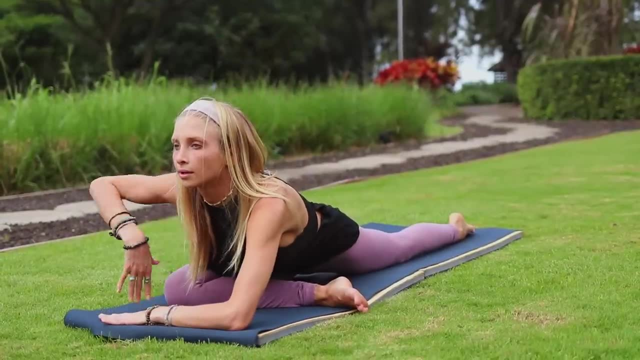 knee to your right thumb, drop your shin to the floor, square out your hips, make sure the back leg is along the center of your mat and then, once you're ready, walk your way over to your elbows. stay there or, if you're comfortable, all the way down with your head to the floor. 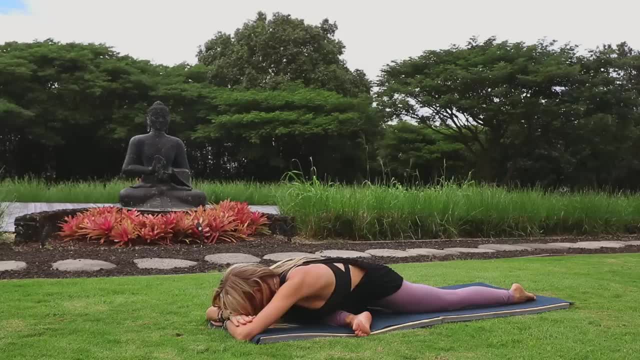 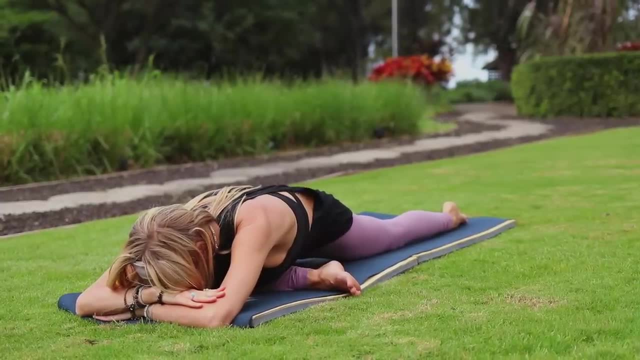 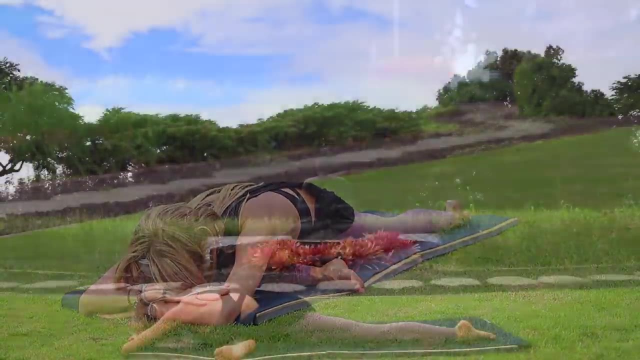 coming into our full pigeon on the mat again. another wonderful posture to help you release any pain like sciatica or soreness in the glutes. so, as you're breathing in your breath, take a deep breath in, then exhale and release. bring all of your awareness to that right glute muscle. 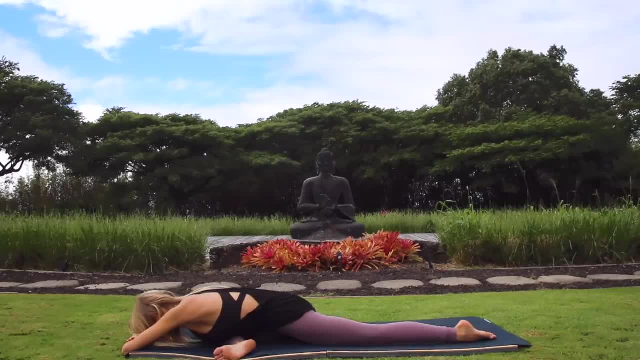 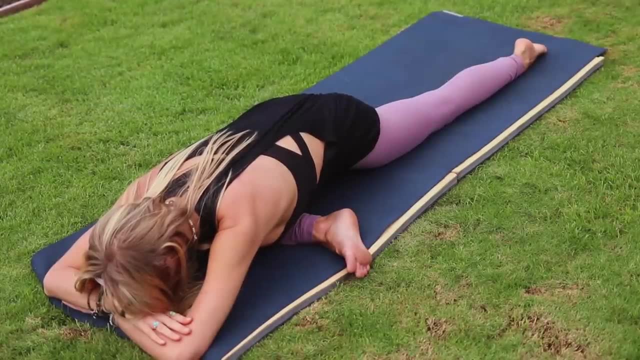 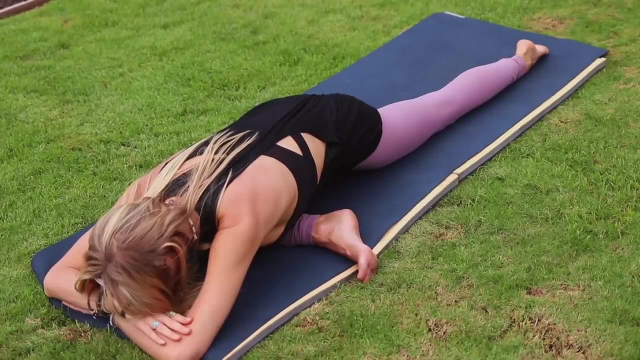 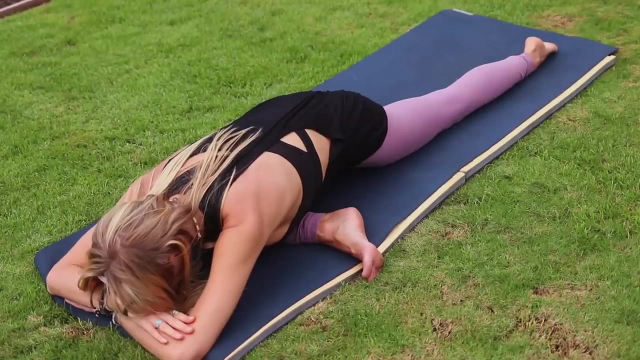 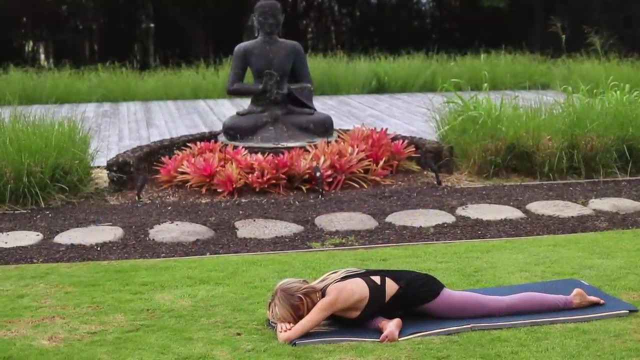 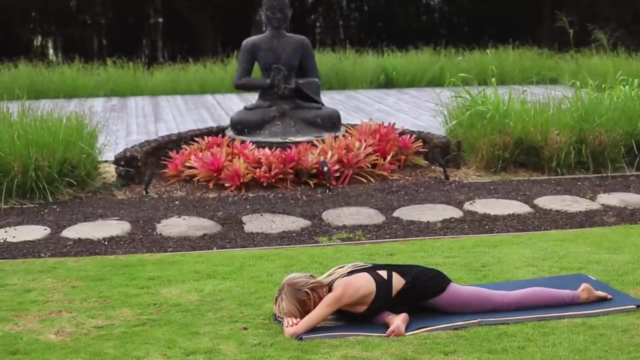 notice where you're feeling that resistance, where is that tension with your inhalation? welcome wonderful, beautiful, healing energy into that area of your body with your exhalation. let go the old, the negative, the past, all that no longer serves you. just let it go. make that choice to exhale and release it out and away from you. 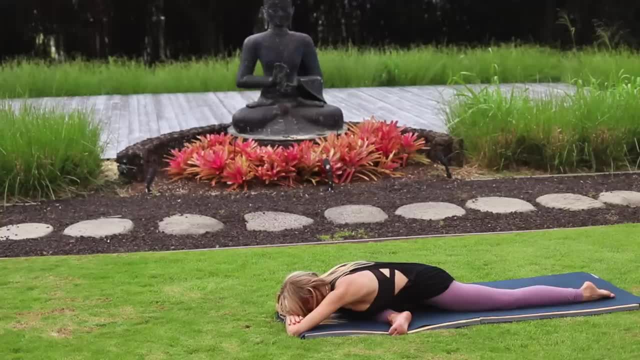 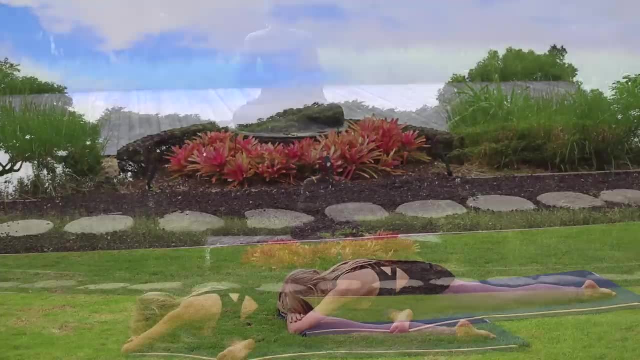 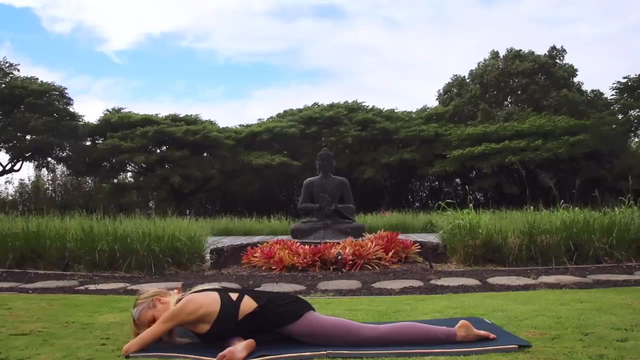 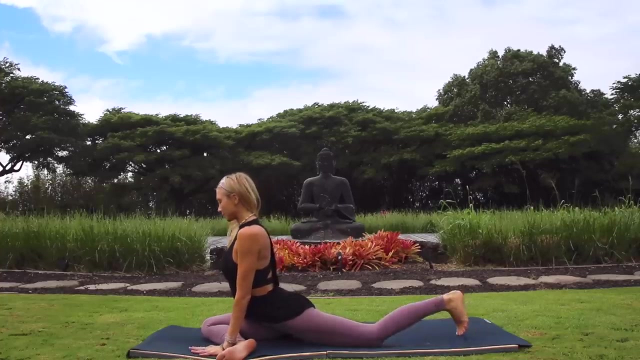 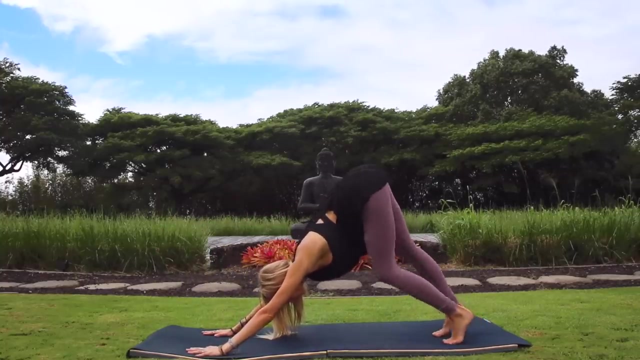 let's take another deep breath in and exhale out slowly. let's begin to bring ourselves up. so come on up to your hands, lift the chest all the way up, tuck your back toes and push yourself right into that downward facing dog, walk it out on the spot. just adding some movement into the legs, into the hips here. 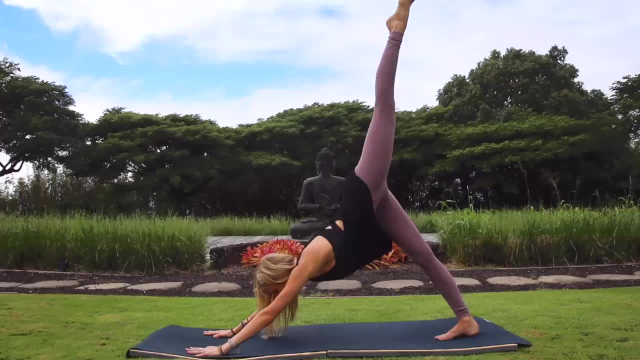 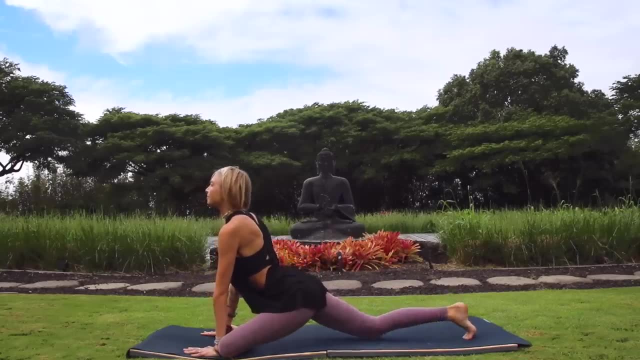 staying in your downward dog. once you're ready, reach the left leg up, bend the knee and bring that left knee now towards your left thumb. square the hips out and walk that back leg all the way back so your hips are square, and then come on over to your 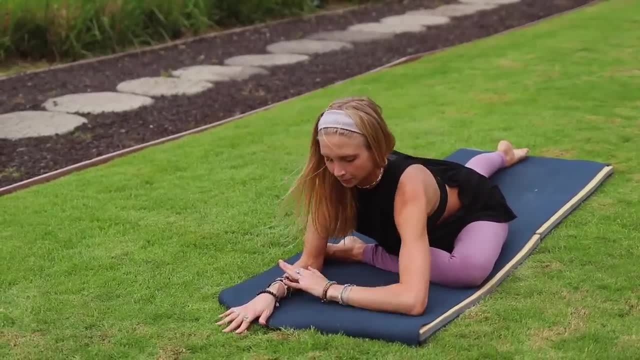 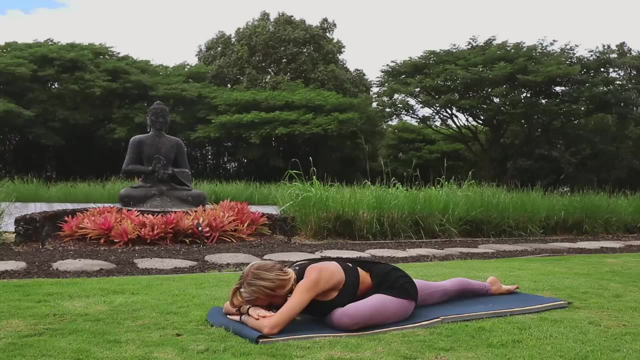 elbows and then all the way down with your chest. if that feels good for you now, you don't need to work your back legs. you don't need to work your back legs. you don't need to work your back legs if your shin is not exactly parallel with the front of your mat. That's not. 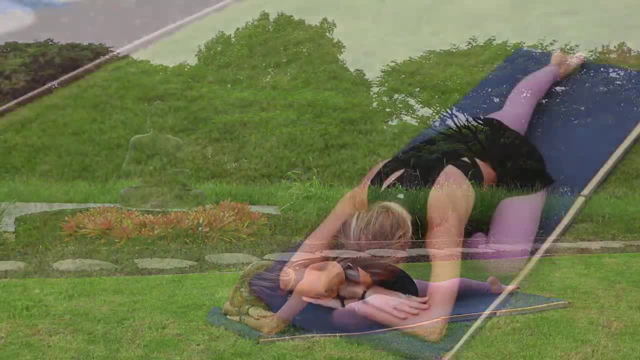 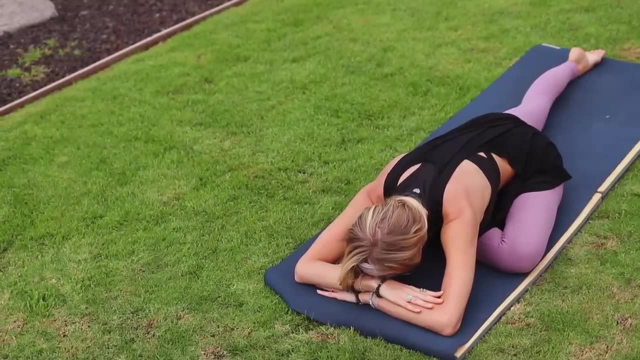 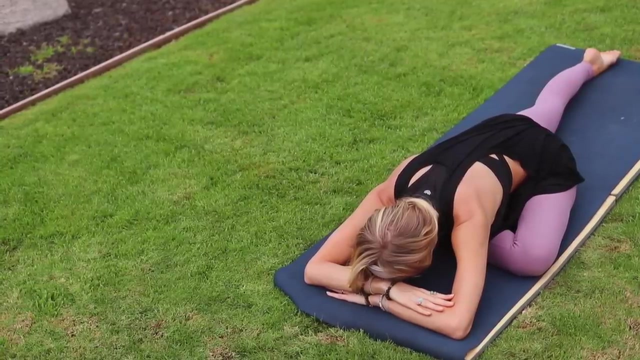 the goal here, Our goal with this particular posture, is to release that glute muscle. So if you are pretty tight here, you might want to keep your left heel closer towards the body, and that's okay. With time, as you release, as your body heals, you will be able to go further and further. But for now just do. 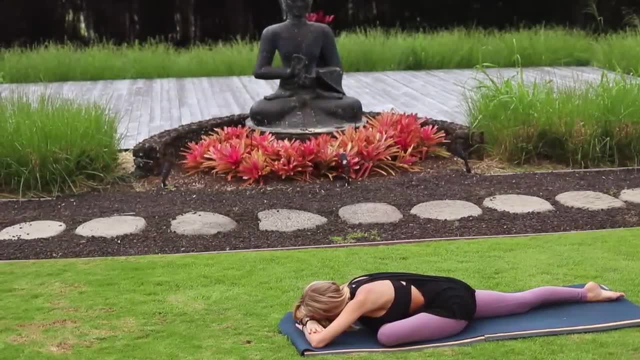 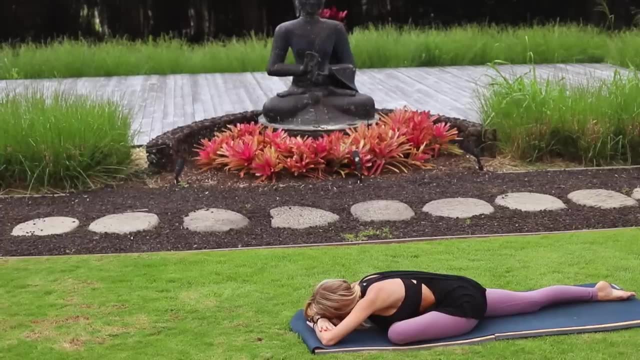 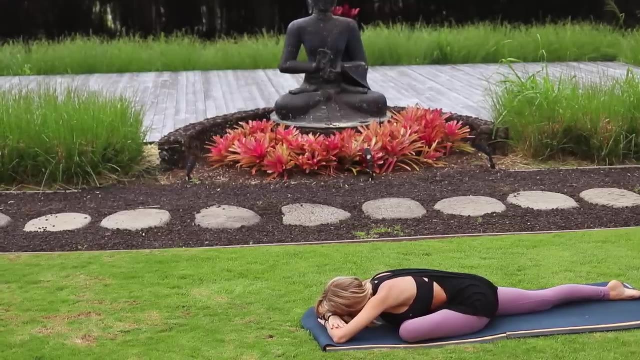 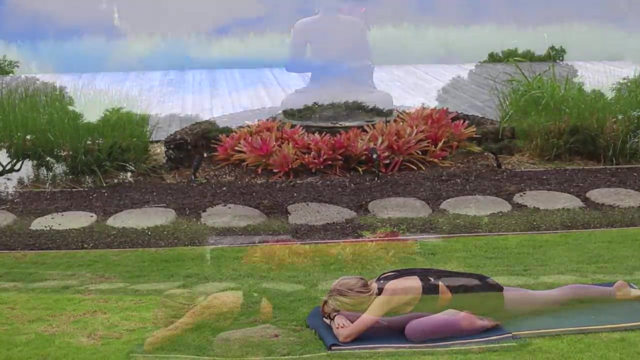 whatever feels comfortable for you: Deep breath in and exhale out. Notice if any emotions arise in this particular posture: Emotions of frustration, anger, sadness, whatever it may be. sometimes we tend to hold on to those energies in our bodies, especially in our hips, in our glutes. 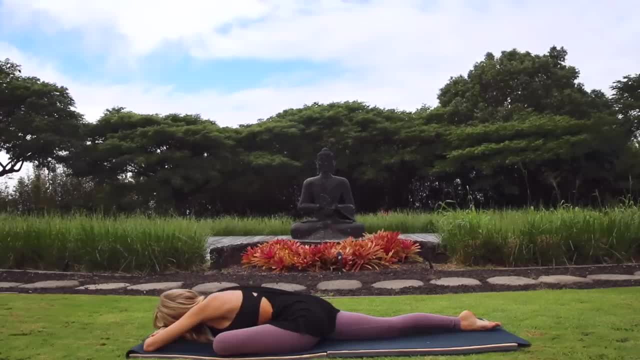 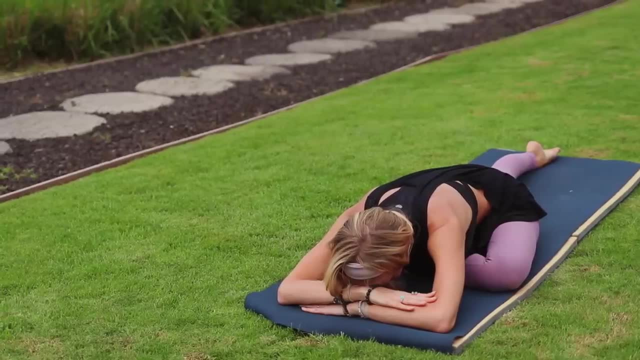 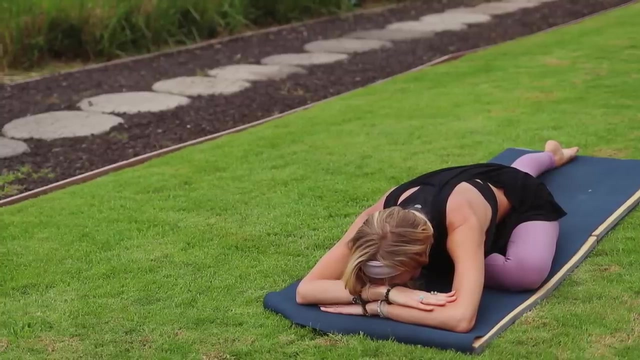 and in our shoulders. So when we target these particular areas of the body, not only are We releasing tension physically, but you're also going to feel an emotional release as well. So if that happens to you, don't hold back. Let it go, Let that. 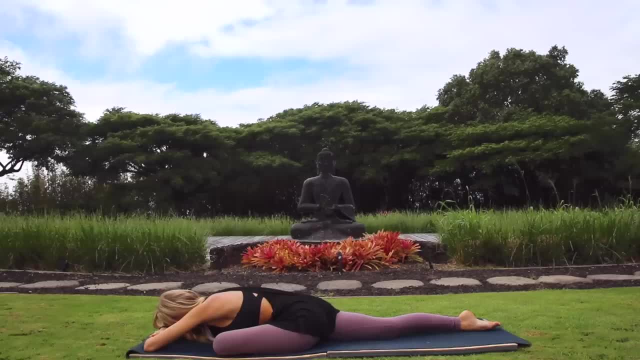 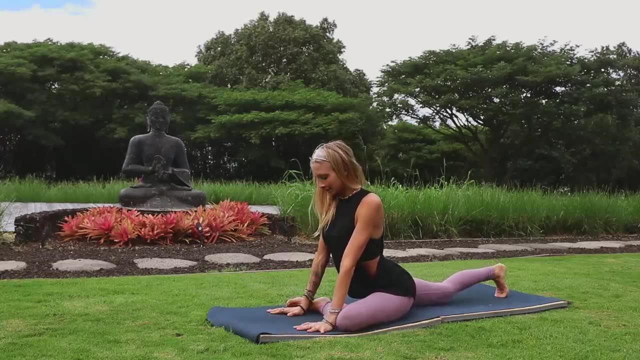 energy release out of you so you can feel lighter and more free. All right, let's slowly Come on out now, up now, ground your hands, tuck your back toes underneath you and, pushing yourself right up into your downward facing dog, walk it out on the spot if that feels. 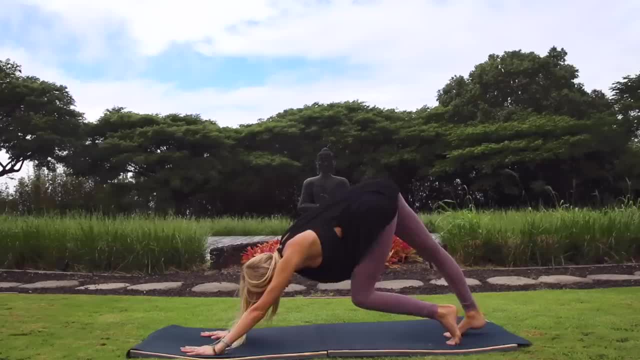 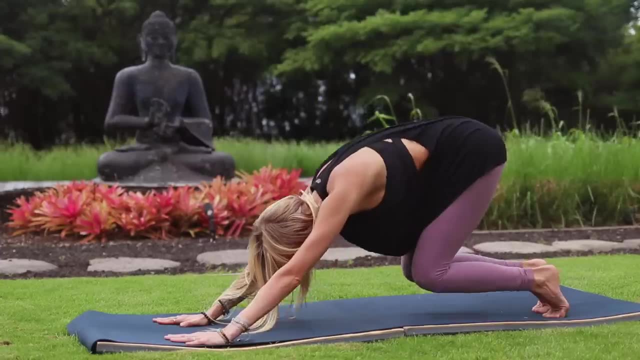 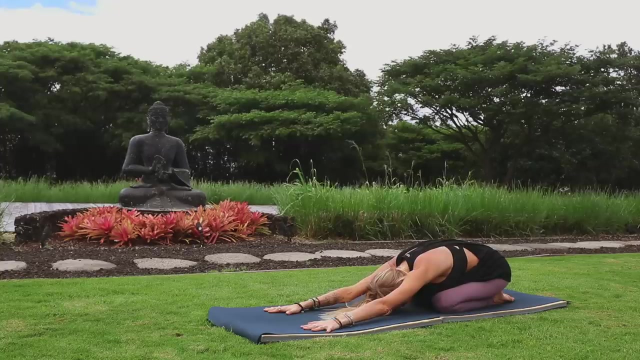 good, deep breath in, exhale out. just add some movement into the hips. feel free to shake out your legs if you have to, and then, once you're ready, bend your knees and sit back into that child's pose one last time, allowing the hands to reach forward or, if you like, to keep them next to the side of your body, that's okay, as. 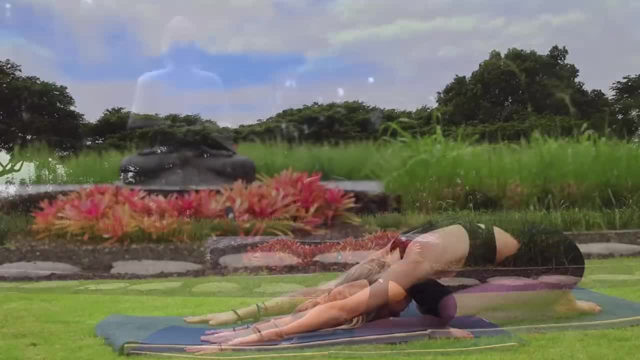 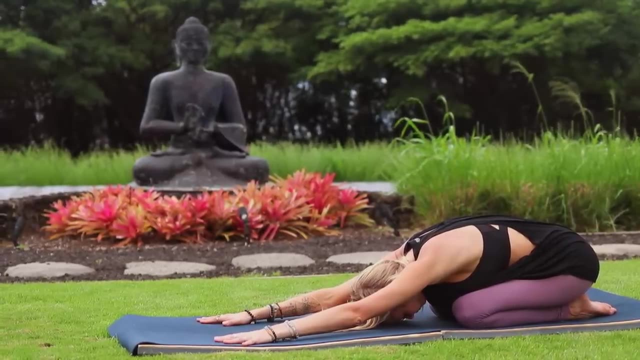 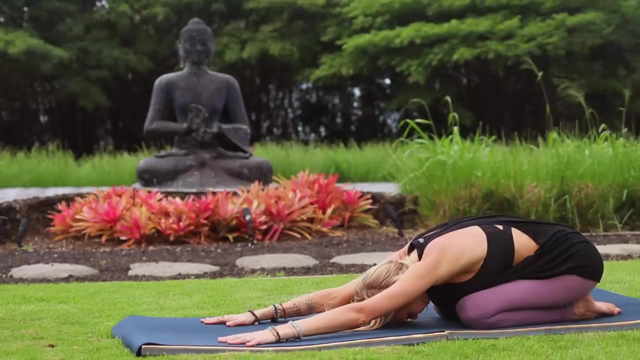 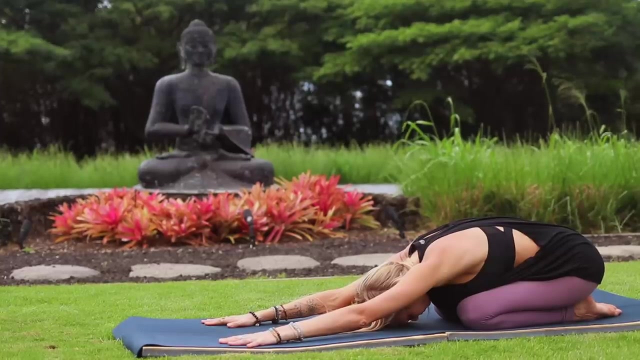 well, allowing the hips to sink right over to your heels, taking a deep breath in and exhale, let it out. check in with your body here. notice how you felt in the beginning of the practice to how you feel right now. bring that awareness into that particular area of your body that's been 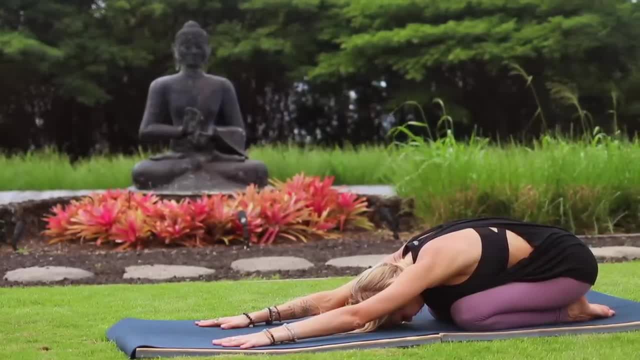 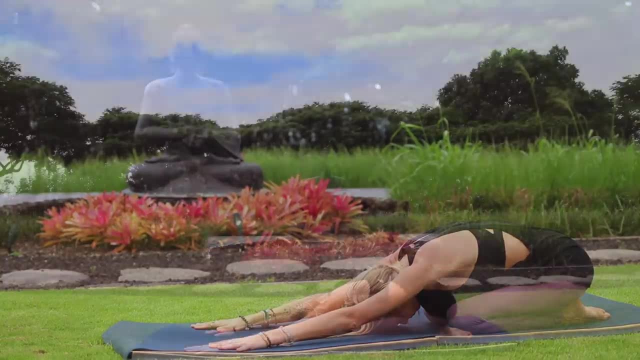 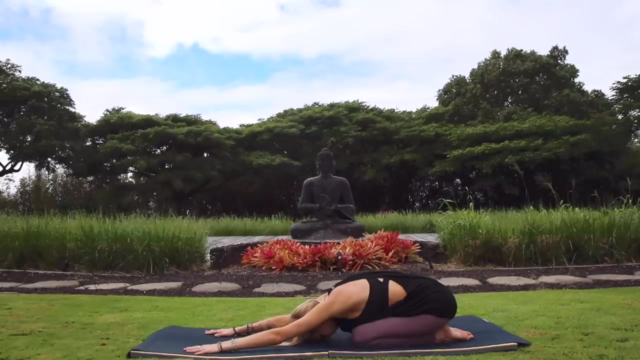 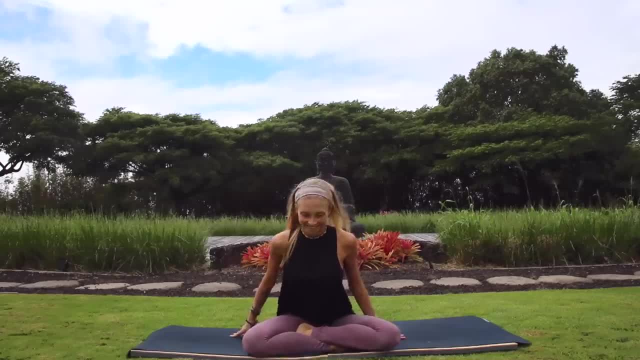 center and just come on over to a center and just come on over to a seated position on your mat, with your feet seated position on your mat, with your feet seated position on your mat, with your feet crossed in front of you. sit up nice. crossed in front of you, sit up nice. 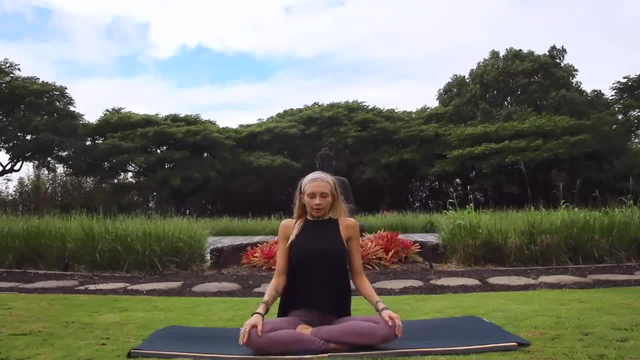 crossed in front of you. sit up nice and tall here, resting your hands on your and tall here, resting your hands on your and tall here, resting your hands on your knees, allowing the shoulders to drop knees, allowing the shoulders to drop knees, allowing the shoulders to drop away from the ears. close your eyes, let's. 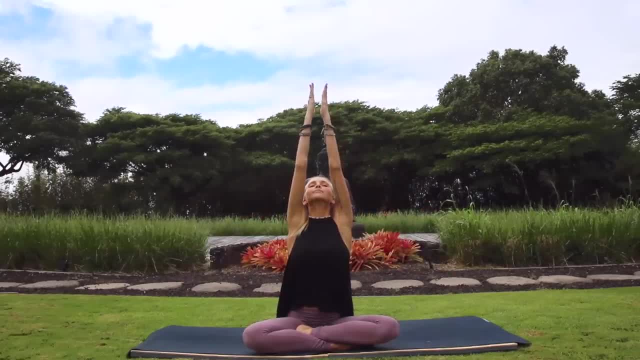 away from the ears. close your eyes. let's away from the ears, close your eyes. let's take an inhale, reaching both arms up to take an inhale, reaching both arms up, to take an inhale, reaching both arms up to the sky. bring the palms of your hands.